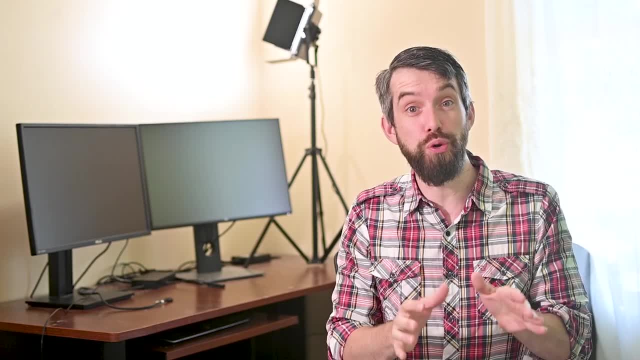 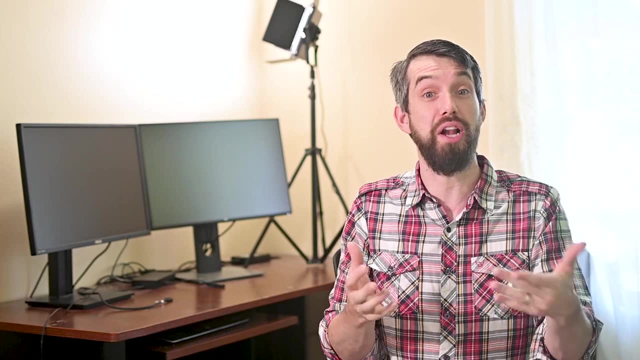 In this video, I'm going to share a bunch of tips on how to prove math theorems, And math theorems can often be a little bit scary and a little bit challenging for students who are just starting out their journey on proving math theorems. Indeed, it's often the case in first and second. 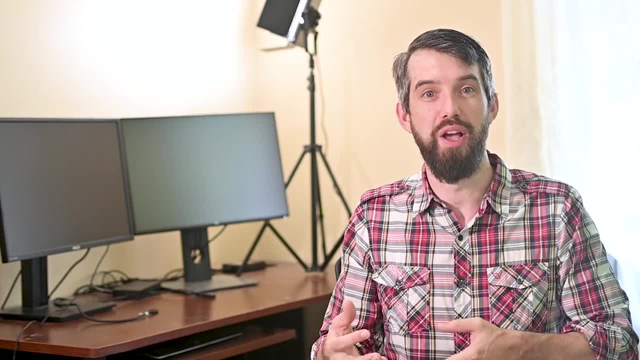 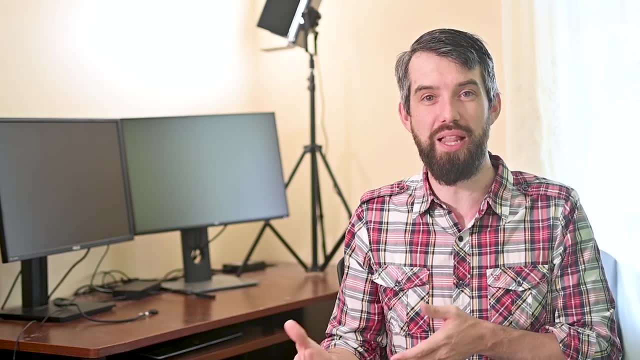 year math courses at university that students are expected to show a lot of procedural fluency with computations, and so when it comes to transition, to be able to prove things, it can be a little bit challenging. So in this video I really want to give you some tools, some ways to scaffold your 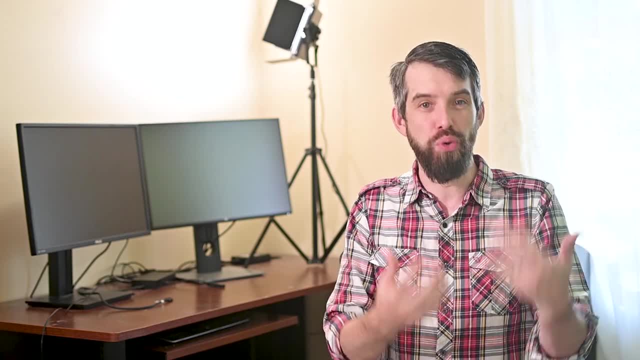 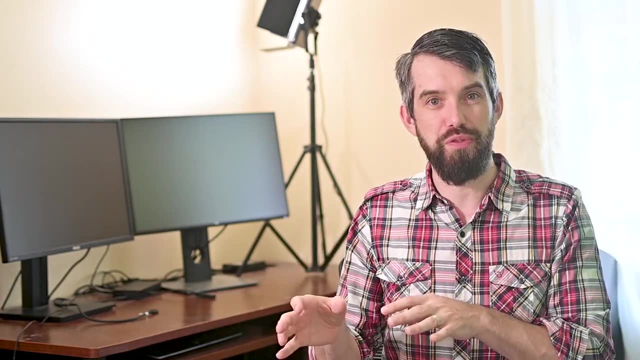 thinking, so that you can at least have some opening moves to get started on whatever it is that you might want to prove. In the first portion of the video, I'm going to focus more on the logic behind different types of proofs, and in the final half of the video I'm going to talk more about. 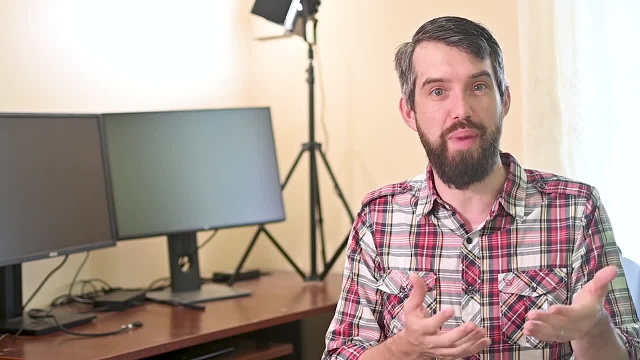 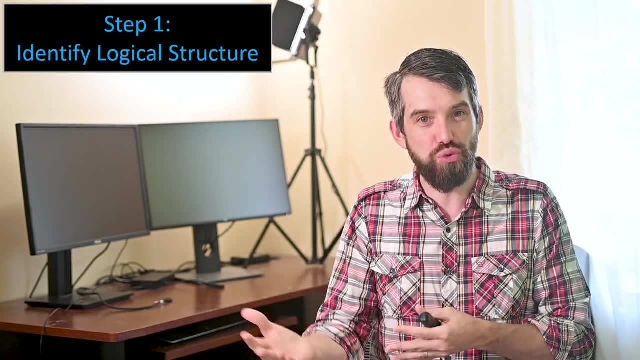 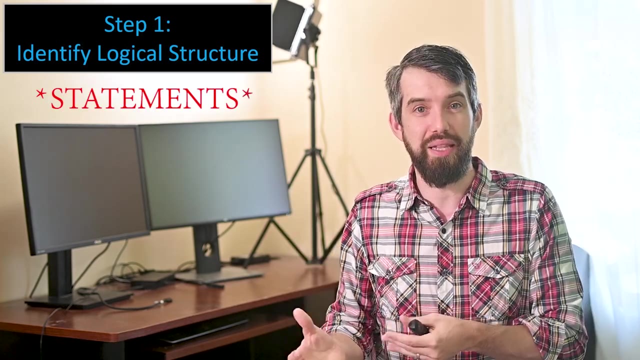 how you come up with the ideas to proceed in your mathematical proof. All right, so step one that I always like to do first is to identify the logical structure of the proof that you want to prove. The most common one that you're going to see is going to be conditional probabilities. 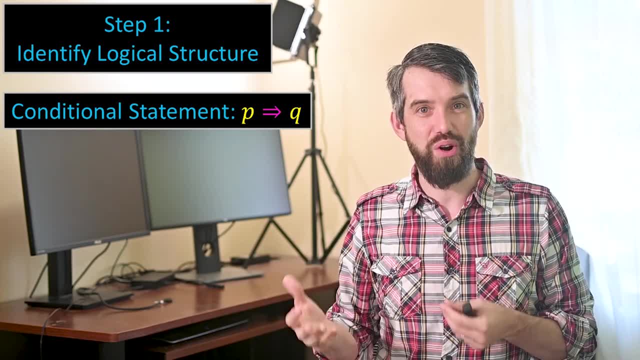 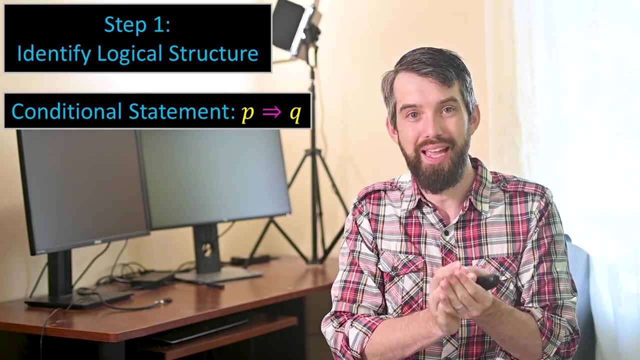 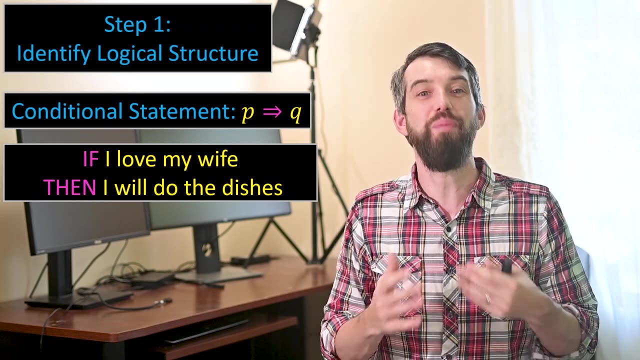 P implies Q. Whenever you see this symbol with this arrow, what it means is that you have some assumptions P and you're trying to prove some conclusion Q. It's an if-then statement. So as an example, I could say: if I love my wife, then I'll do the dishes, or something like this. 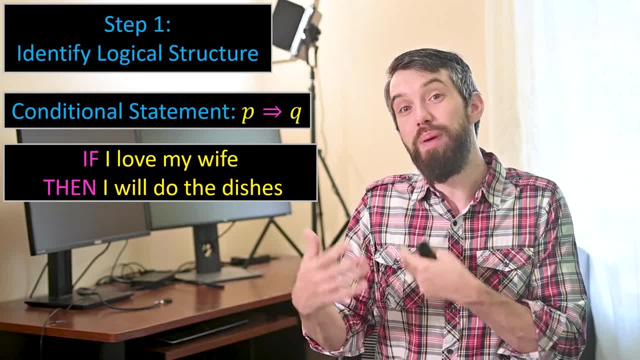 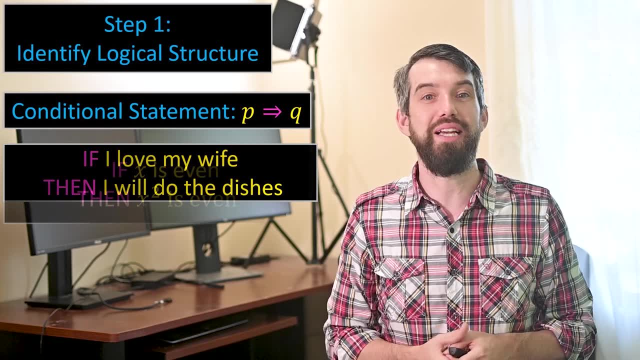 It's got an assumption and it's got a conclusion, And this basic structure is there regardless of the actual details of the assumption, the details of the conclusion. So, for example, consider this claim: If X is an even number, then X squared is an even number. 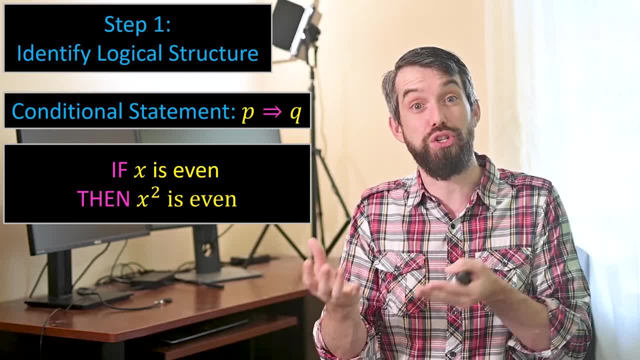 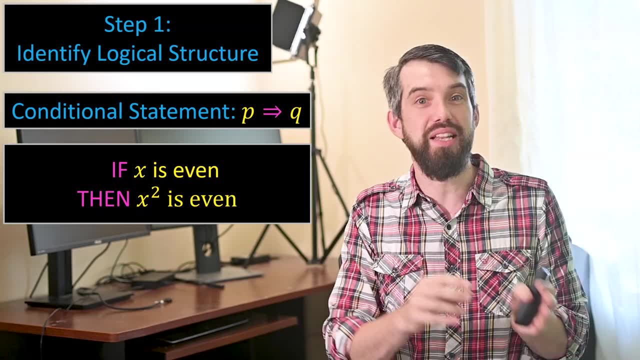 That is also a mathematical claim. that is also in the structure of a conditional statement And often proofs aren't written quite so clearly as an if, some assumptions, then some conclusions. We may have sort of turned the words around, but if you can take whatever is given and interpret it, 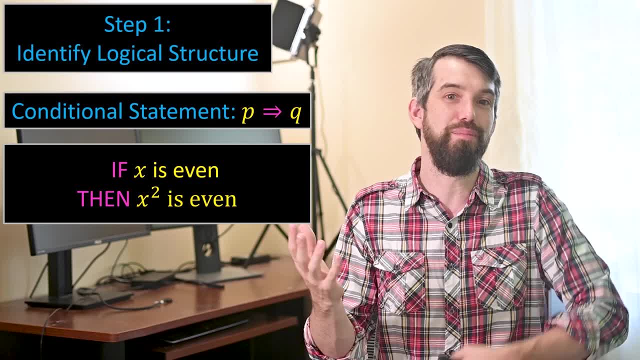 in this way where you've got an assumption and you're trying to prove something and you can take whatever is given and interpret it in this way, where you've got an assumption and you've got an assumption and a conclusion and it's saying: if the assumption, then the conclusion, 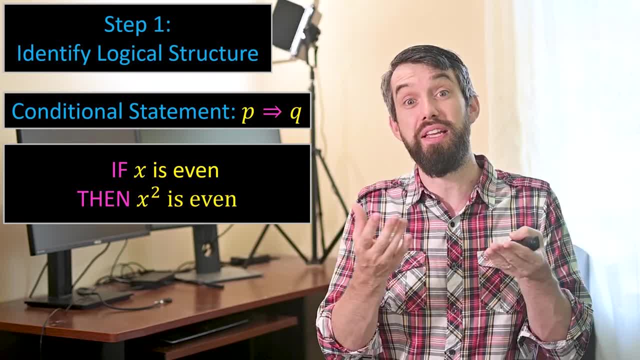 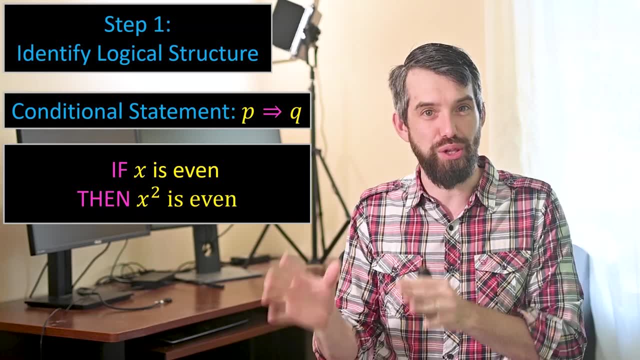 also a mathematical claim that is also in the structure of a conditional statement And often proofs aren't written quite so clearly as an if, some assumptions, then some conclusions. We may have sort of turned the words around, but if you can take whatever is given and interpret it in, 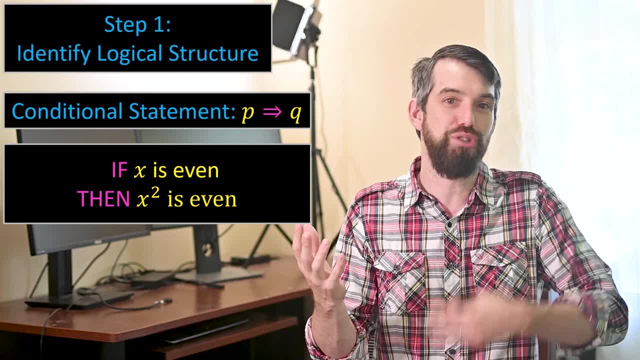 this way, where you've got an assumption, then that is also a mathematical claim. Now, if you're looking at the words that you're going to keep and setting up, on them, of course there's people who and a conclusion and it's saying: if the assumption, then the conclusion, then that's going to be very useful for coming up with a strategy to actually prove this claim. 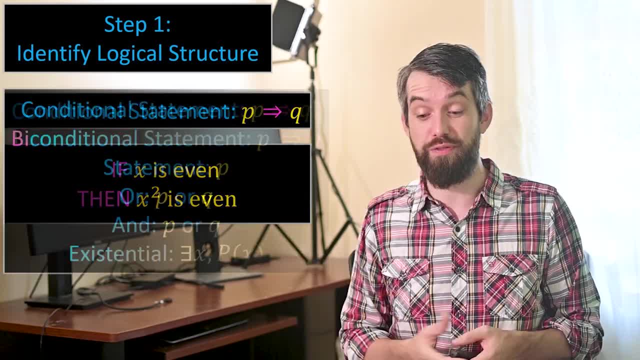 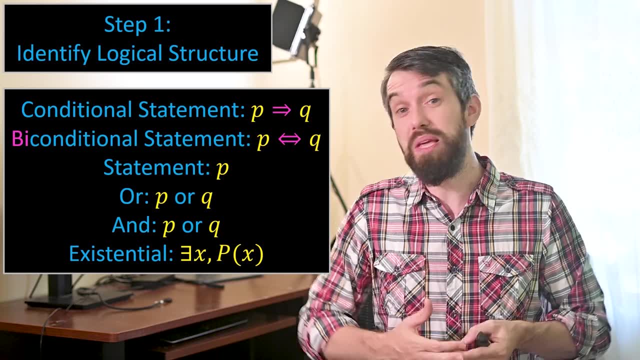 Now, conditional statements are not the only type of statements. I have to put up a list of a bunch of different types of possible logical structures that your claim has. It might, for example, the second line be a biconditional. Biconditionals are interesting because they're kind of like two different conditions at the same time. 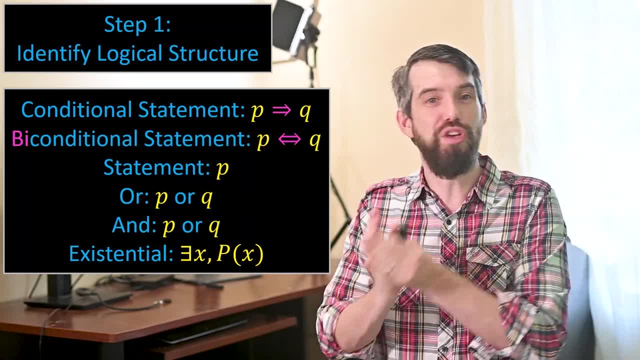 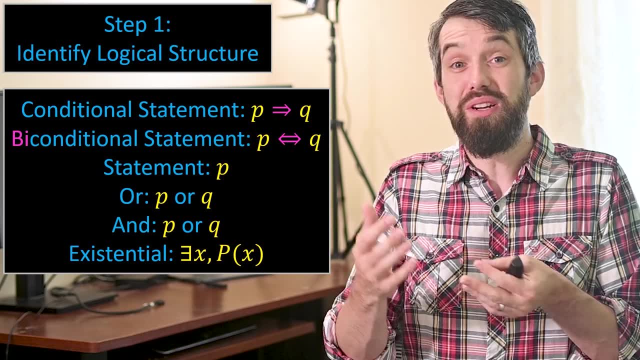 You're saying if P then Q, and if Q then P. If you have a biconditional, you have really two proofs that you have to do, showing the one direction and the other. Sometimes, however, it's not structured as a statement, like, for example, the claim there are infinitely many prime numbers. 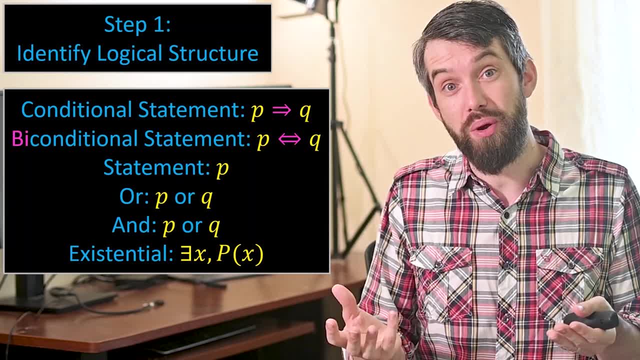 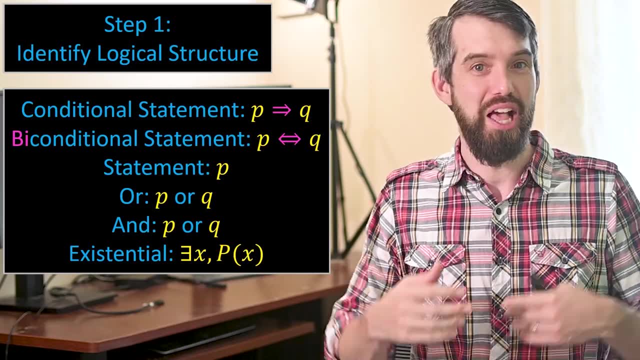 Sometimes you have a P and a Q, or a P or a Q, And sometimes you have structures where what you're really trying to do is show that there exists- this is what the backwards E means- there exists some value that obeys some. 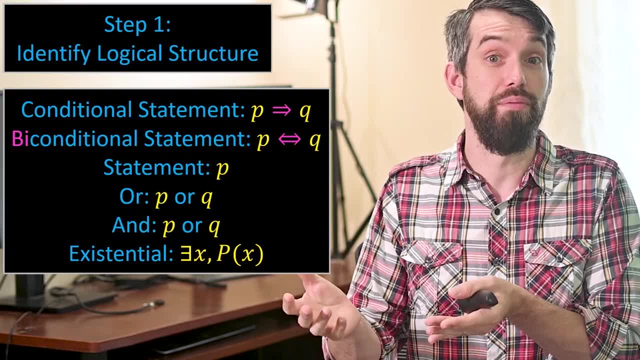 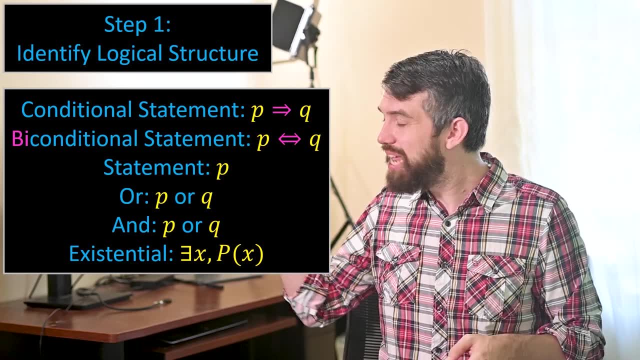 Properties. An example of this might be: like there exists an oldest human on planet Earth. Okay, so after you've analyzed the sort of logical structure and try to figure out what you're doing, the next step would be to try to figure out: well, what method are you going to use to prove it? 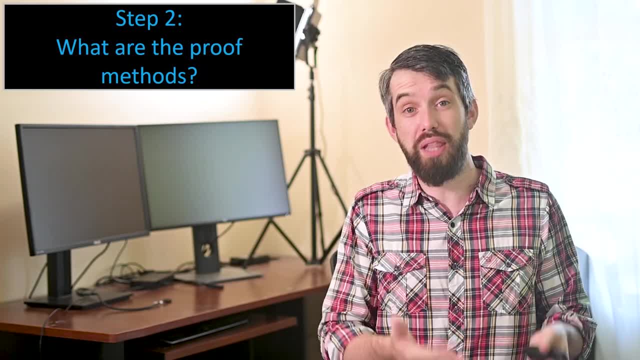 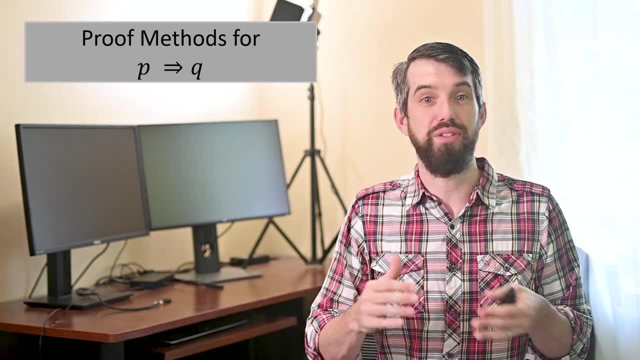 And there's actually a bunch of different methods and it depends on what the structure of the claim was. So, going to the most common one, the proof methods for a conditional, and if P, then Q. Well, it turns out there's a bunch of different methods that you can use to prove a conditional. 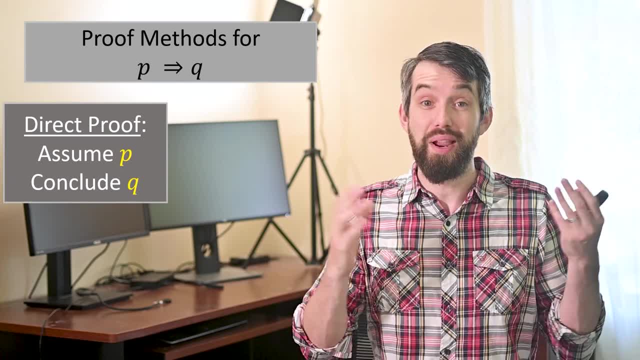 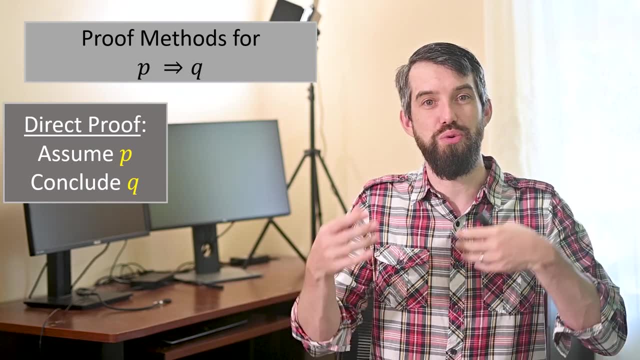 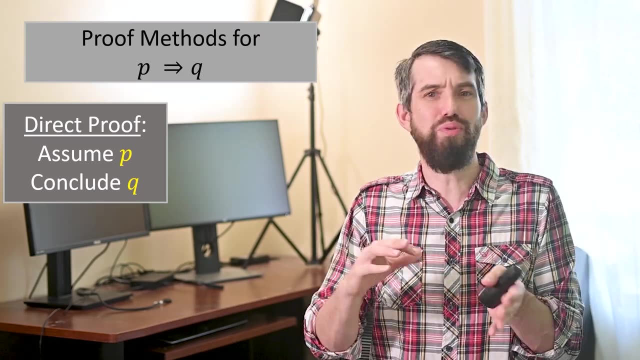 The most sort of direct one is well uninspiringly called a direct proof. It says: just assume the assumption which is P, and then you do some sort of manipulations until you have managed to conclude the conclusion Q. You just basically start at the assumptions and move directly towards the conclusions and probably the most common proof structure you'll see. 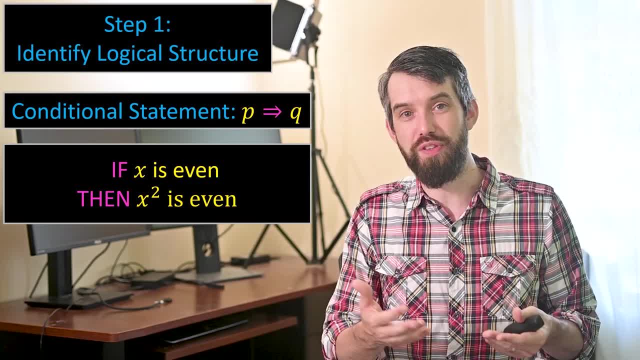 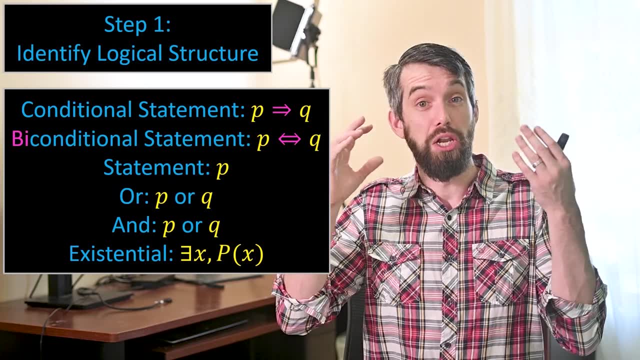 then that's going to be very useful for coming up with a strategy to actually prove this claim. Now, conditional statements are not the only type of statements. I have to put up a list of a bunch of different types of possible logical structures that your claim has. It might, for example, 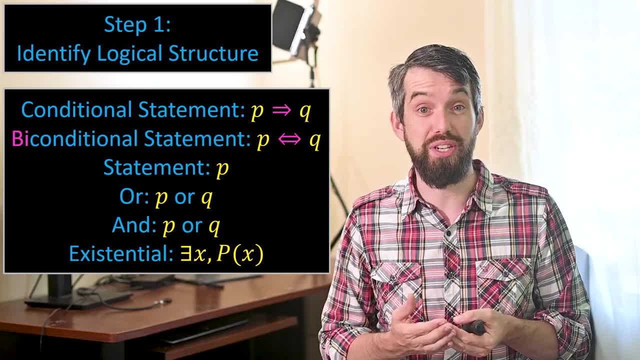 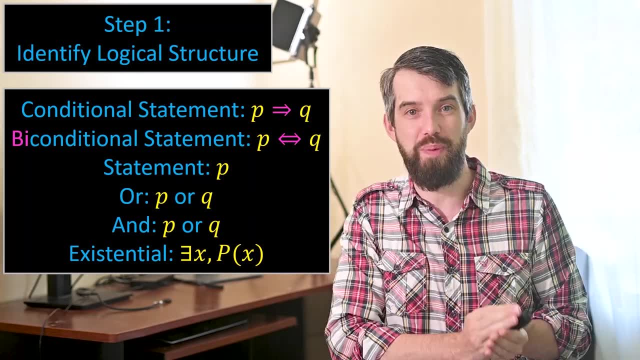 the second line be a biconditional. Biconditionals are interesting because they're kind of like two different conditions at the same time. You're saying: if P, then Q, and if Q then P. If you have a biconditional, you have really. 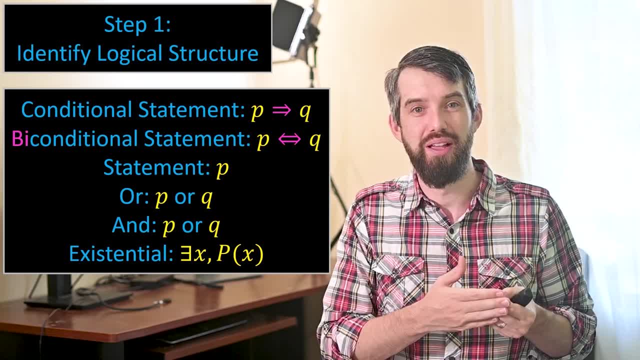 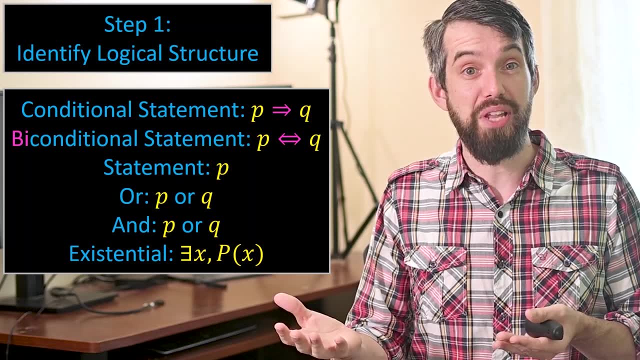 two proofs that you have to do, showing the one direction and the other. Sometimes, however, it's not structured as a statement, Like, for example, the claim there are infinitely many prime numbers. Sometimes you have a P and a Q, or a P or a Q. 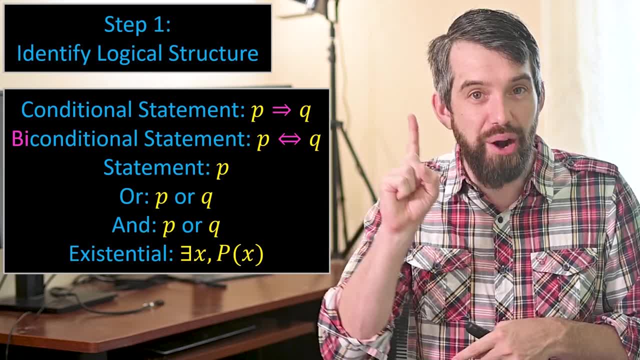 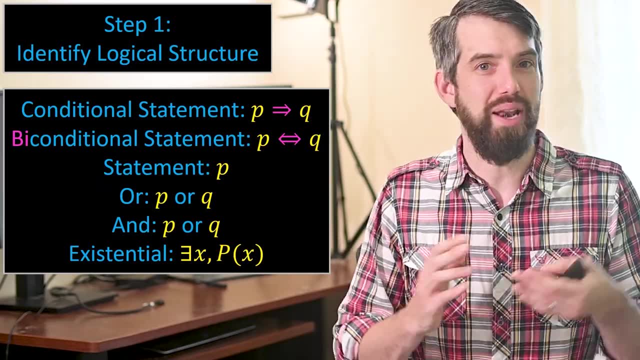 And sometimes you have structures where what you're really trying to do is show that there exists. this is what the backwards E means: there exists some value that obeys some properties. An example of this might be like there exists an oldest human on planet Earth. Okay so. 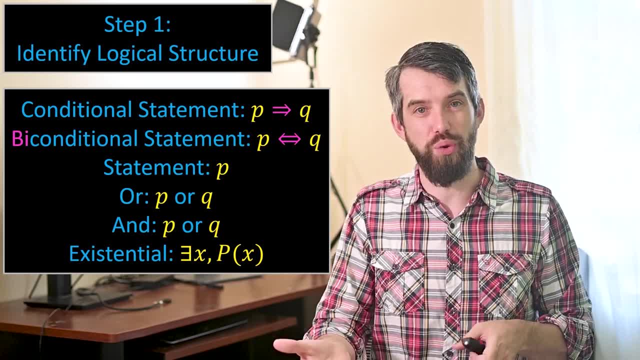 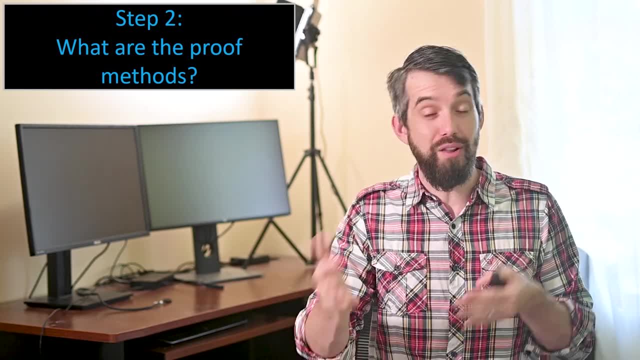 after you've analyzed the sort of logical structure and trying to figure out what you're doing, the next step would be to try to figure out: well, what method are you going to use to prove it? And there's actually a bunch of different methods and it depends on what. 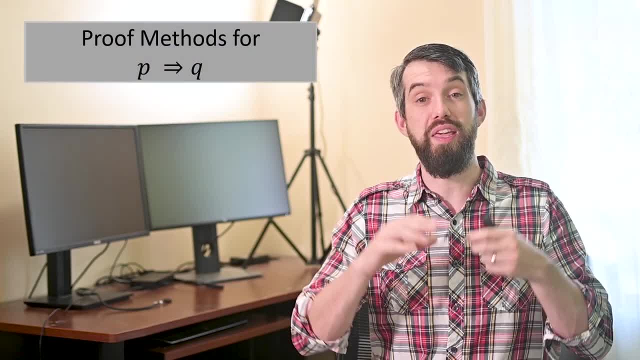 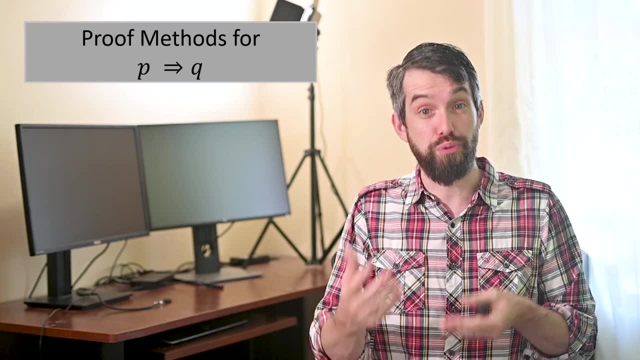 the structure of the claim was So going to the most common one, the proof methods for a conditional. if P, then Q. Well, it turns out there's a bunch of different methods that you can use to prove a conditional like this. The most sort of direct one is: well. 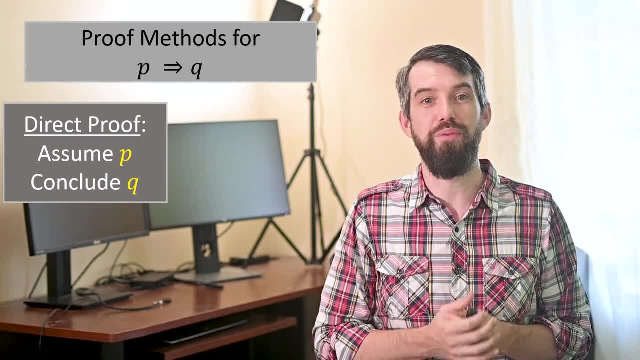 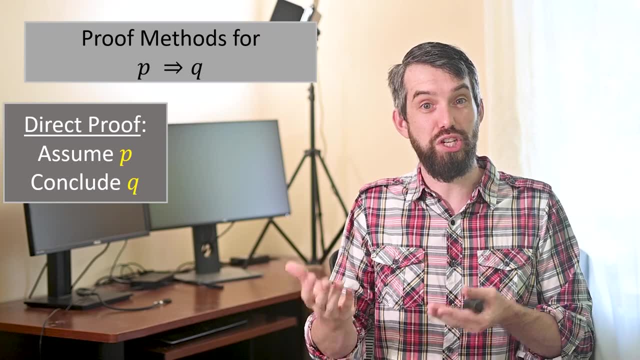 uninspiringly called a direct proof. It says: just assume the assumption which is P, and then you do some sort of manipulations until you have managed to conclude the conclusion Q. You just basically start at the assumptions and move directly towards the conclusions and probably the most common proof structure. you'll see. 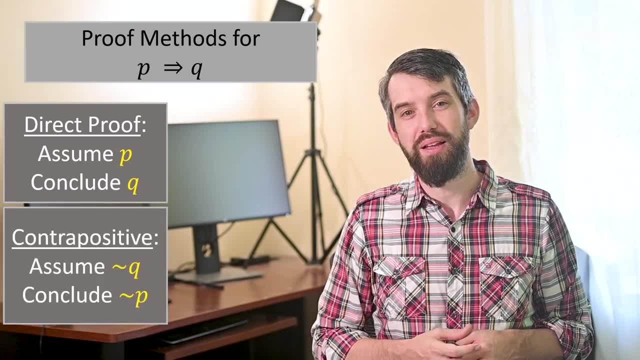 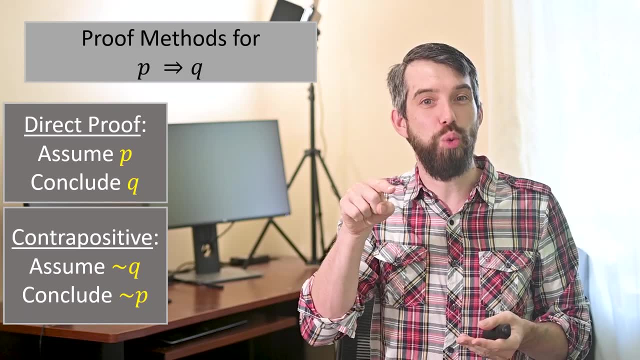 But there's others. For example, there's the contrapositive. Contrapositive goes the other way around. It says: let me assume that the conclusion is false. That is, let me assume, not Q. This little squiggle here means not. So let me assume the conclusion is false. 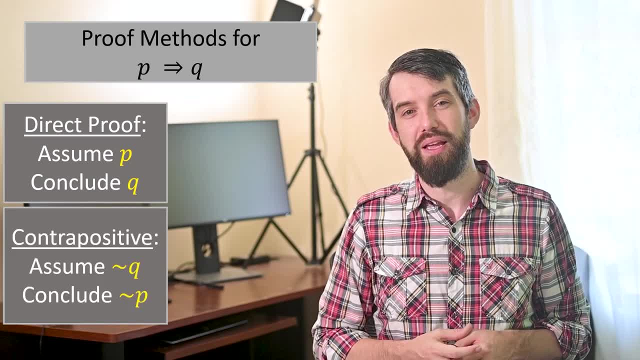 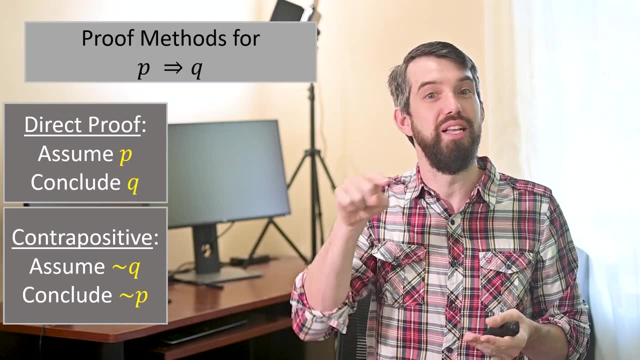 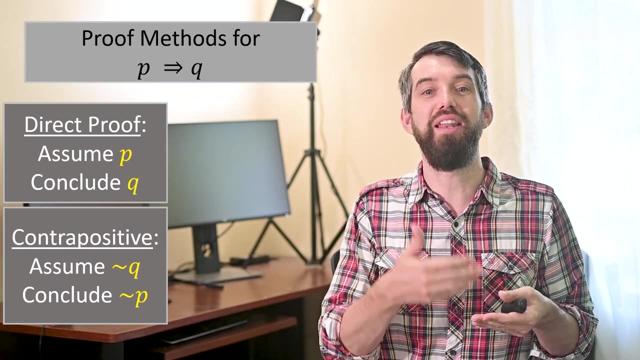 But there's others. For example, there's the contrapositive. Contrapositive goes the other way around. It says: let me assume that the conclusion is false. That is, let me assume, not Q. This little squiggle here means not. So let me assume the conclusion is false. and then I'll continue to do some manipulations until I can finally conclude the negation of the assumption. 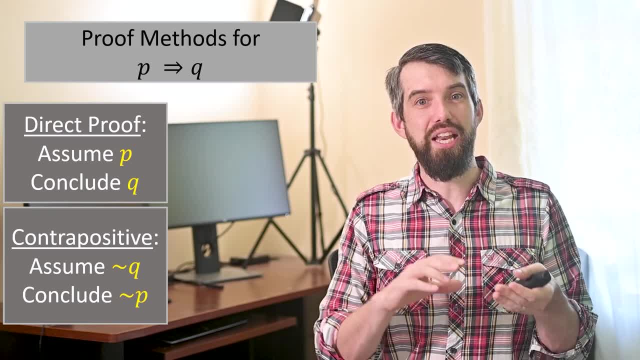 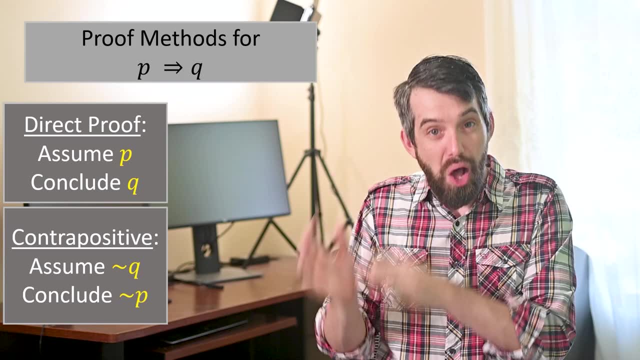 That is, I want to conclude, not P Indeed going. the contrapositive for the claim that if X is even, X squared is even would be that X squared is not even implies that X is not even, And indeed both of these are logically equivalent. It doesn't matter what you do. 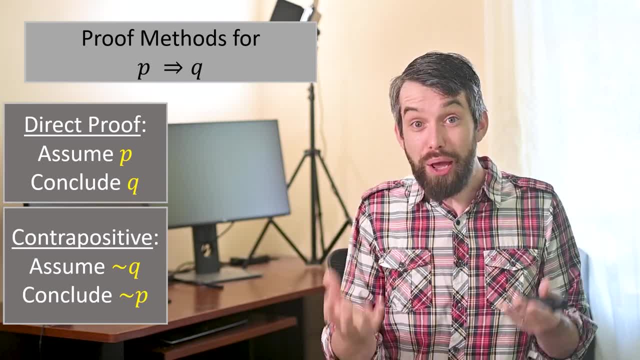 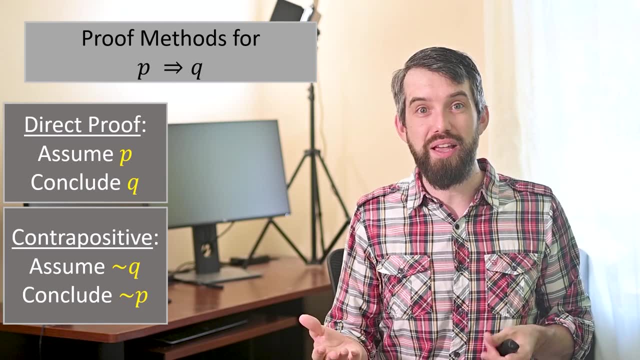 But one of them might be easier for you. So they're both logically the same, but you might have a preference for them based on the complications in the manipulations that you need to do. Another method that's common is the method of contradiction. 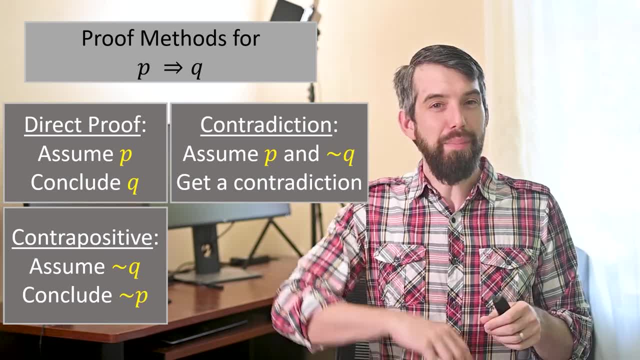 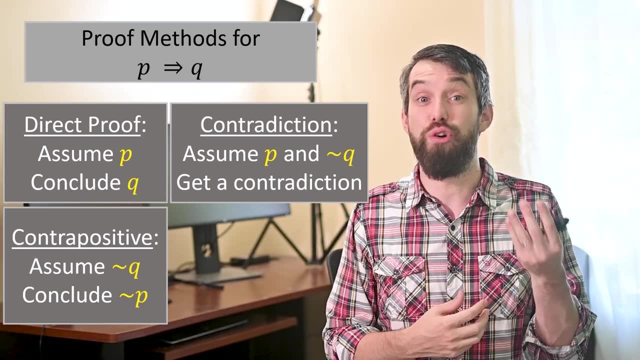 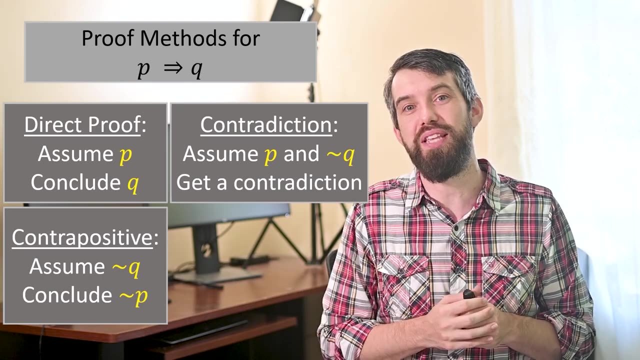 And it says: I have my assumption P already. but let me also assume that my conclusion is false. And if you do some manipulation where you're taking this initial assumption P and you're assuming the conclusion is false and you get some nonsense like zero is equal to one or X is even and odd at the same time, 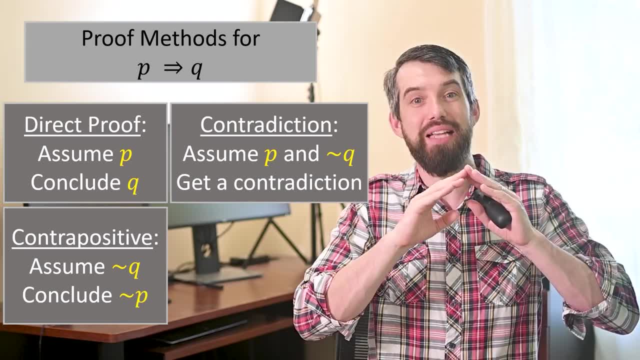 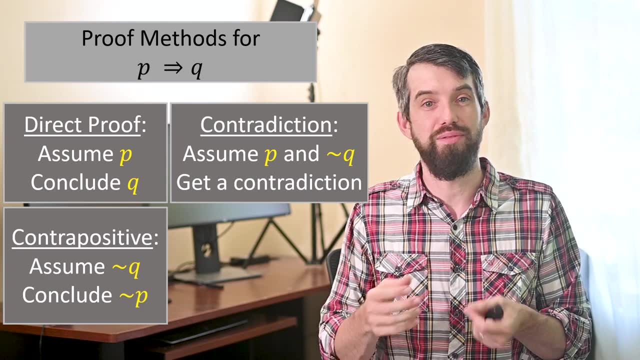 or something is literally independent and dependent at the same time. if you get some contradiction like this, then it must be your assumption: the not Q could not have been the case, And so that is another method to be able to prove things. 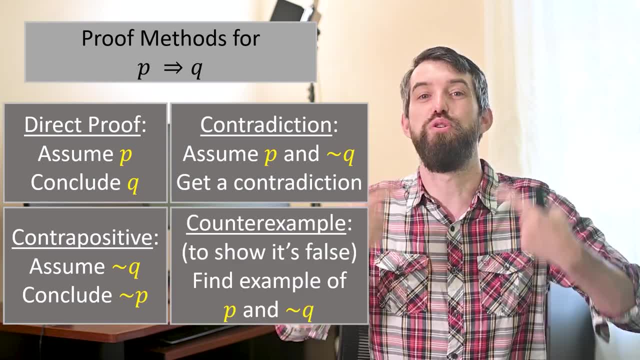 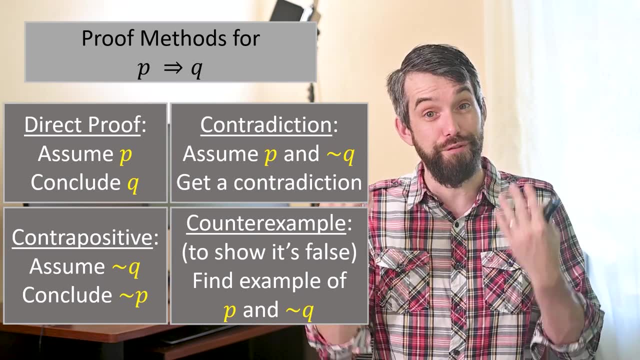 And then the final method is actually not when you want to prove something, It's when you want to prove a conditional is false, And that's the method of counter-example. So this is not me proving P implies Q, It's me showing that P implies Q is false. 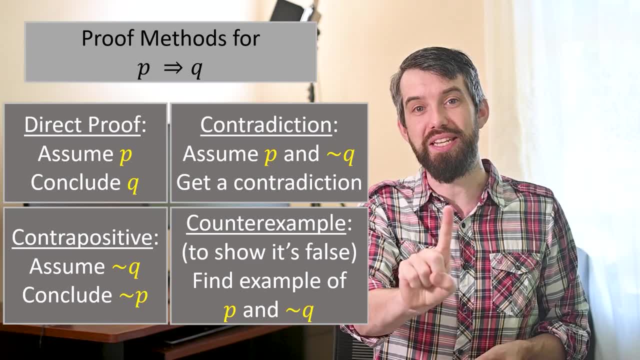 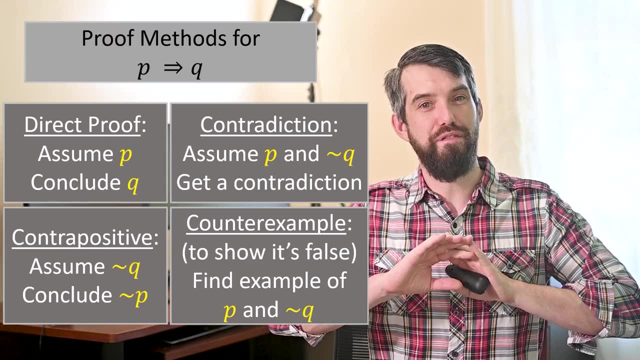 Well, for a counter-example, I just need to give you one example, one instance where the assumption is true, The assumption is satisfied, but the conclusion is not, And it's important to note that counter-example is really quite fundamentally different from the other three. 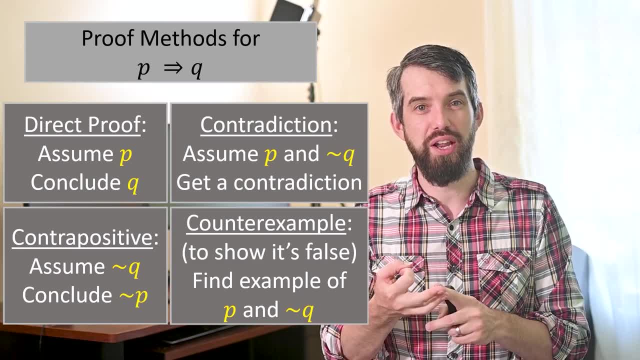 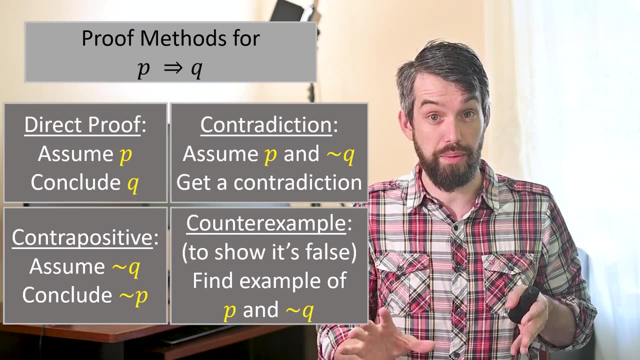 This is because for the direct proof and counter-positive and contradiction, we're showing them in complete generality, But for counter-example we can just use one specific, concrete example. That's sufficient. Indeed, one of the most common errors that I see as a professor who grades people trying to do proofs, 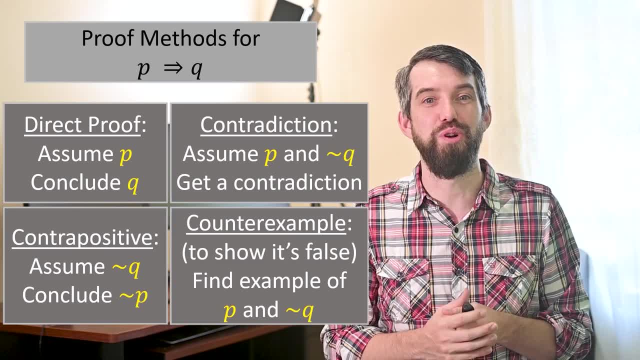 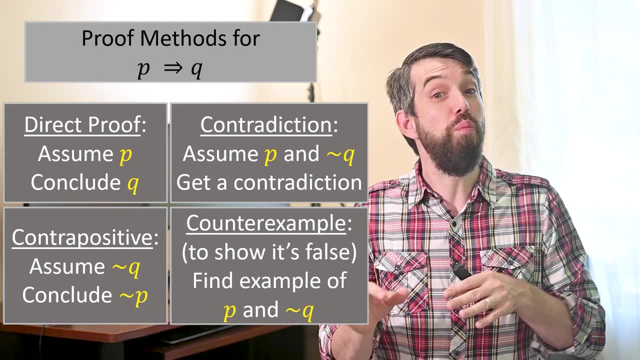 is where someone does a proof by example and they try to do a direct proof and they show it's true in one example, but not show it is true in all examples, And so that's a very important distinction. Now, to be fair, you might not know which of these methods you need to begin with. 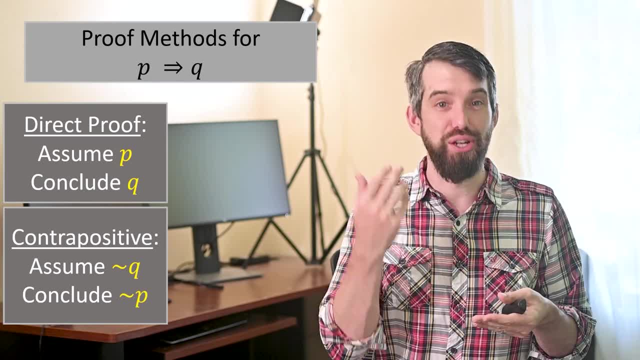 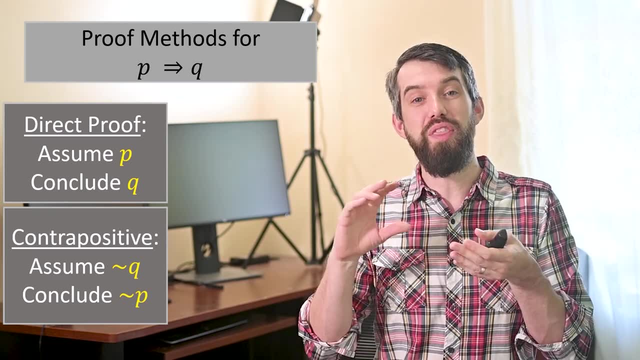 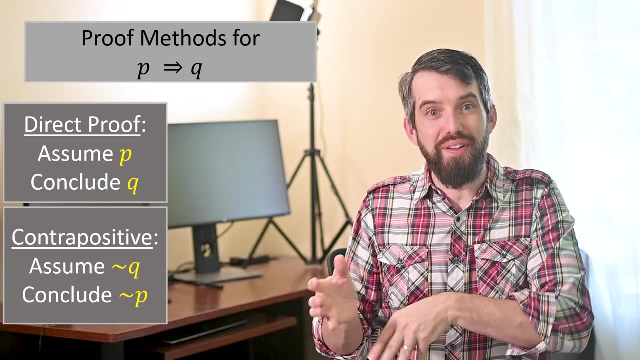 and then I'll continue to do so- Manipulations- until I can finally conclude the negation of the assumption That is. I want to conclude, not P Indeed going. the contrapositive, for the claim that if X is even, X squared is even, would be that X squared is not even implies that X is not even, And indeed, 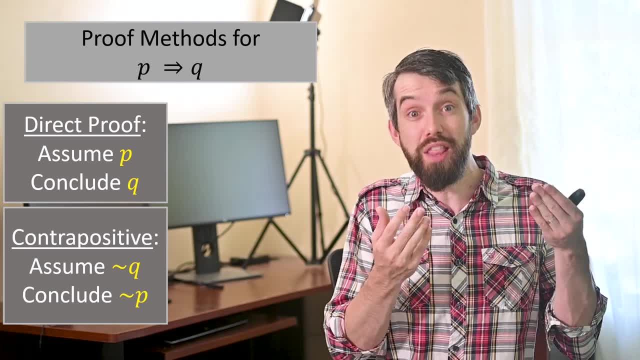 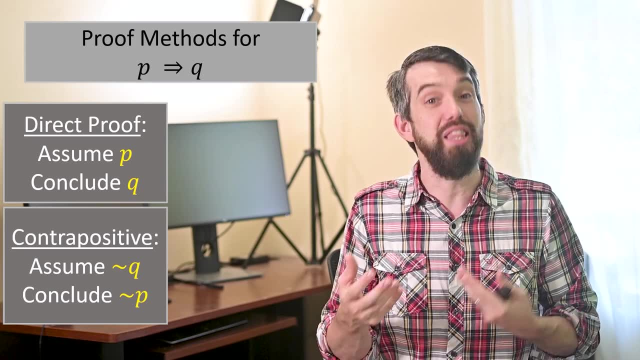 both of these are logically equivalent. It doesn't matter which you do, but one of them might be easier for you than the other. So they're both logically the same, but you might have a preference for them based on the complications in the middle. So let me assume that X is not even. 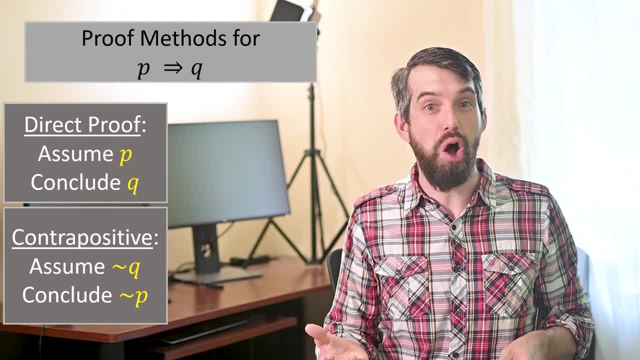 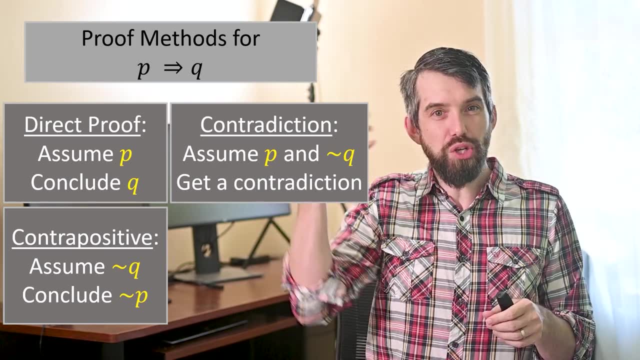 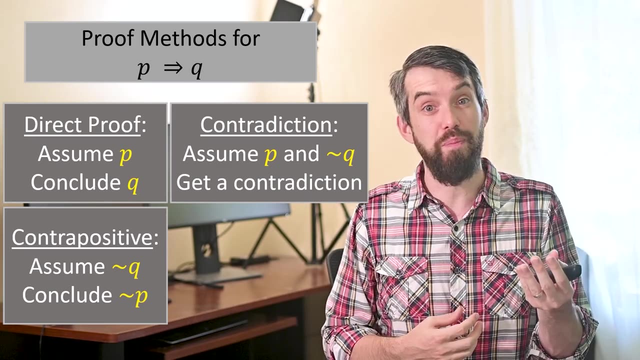 Manipulations that you need to do. Another method that's common is the method of contradiction And it says: I have my assumption P already. but let me also assume that my conclusion is false And if you do some manipulation where you're taking this initial assumption P and you're assuming the conclusion, 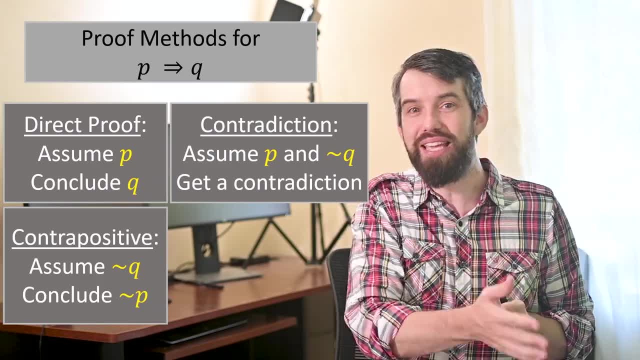 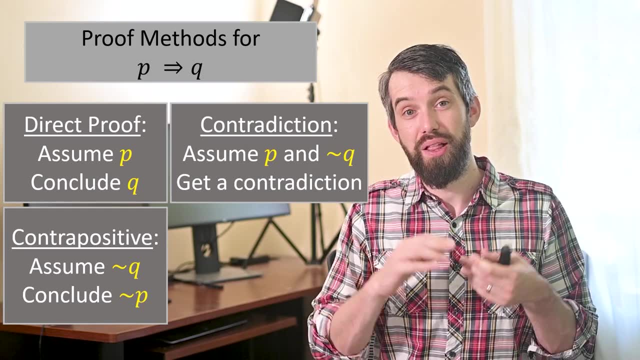 is false and you get some nonsense like zero is equal to one, or X is even and odd at the same time, or something is literally independent and dependent at the same time. if you get some contradiction like this, it must be your assumption. the knock Q. 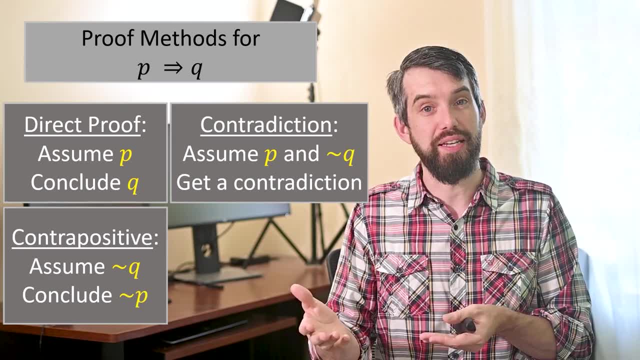 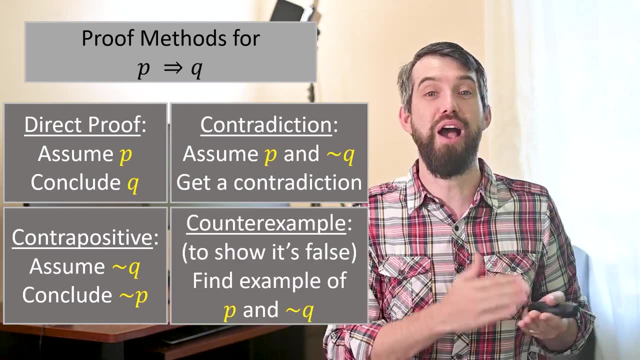 could not have been the case, And so that is another method to be able to prove things. And then the final method is actually not when you want to prove something. it's when you want to prove a conditional is false, And that's the method of counterexample. 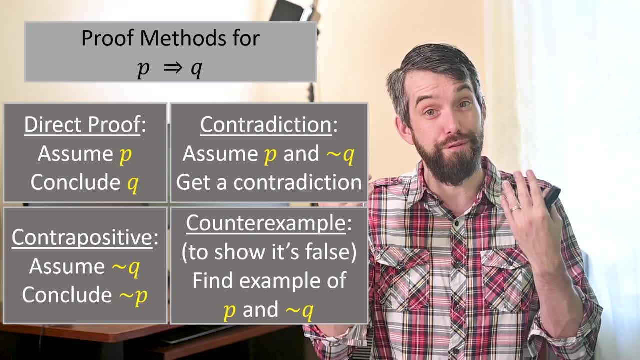 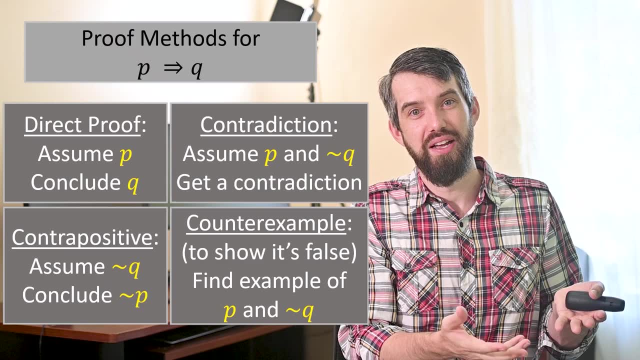 So this is not me proving P implies Q. it's me showing that P implies Q is false. Well, for a counterexample, I just need to give you one example, one instance where the assumption is satisfied but the conclusion is not. 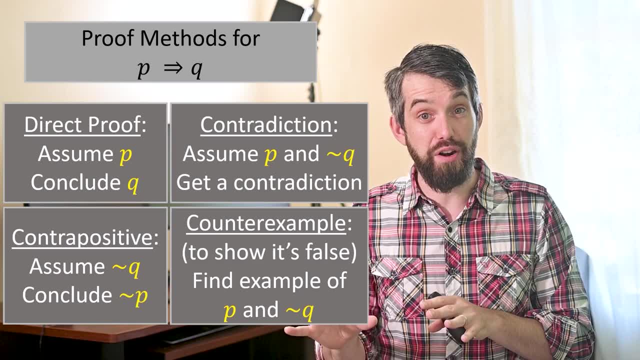 And it's important to note that counterexample is not just conscious of the contradiction, in fact that counterexample is really quite fundamentally different from the other three. This is because for the direct proof and counterpositive and contradiction, we're showing them in complete. 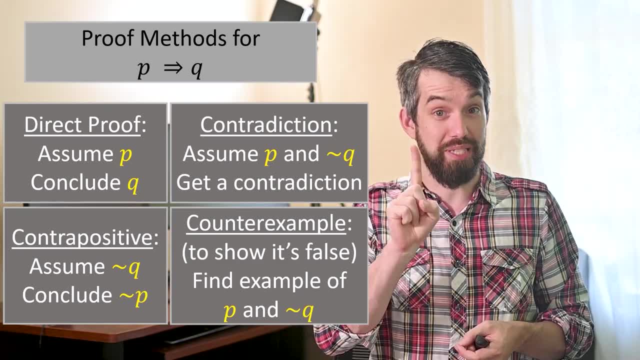 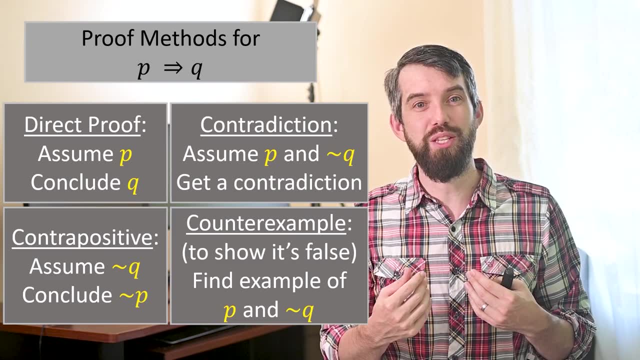 generality, But for counterexample we can just use one specific, concrete example. That's sufficient. Indeed, one of the most common errors that I see, as a professor who grades people trying to do proofs, is where someone does a proof by example and they try to do a direct proof and they show. 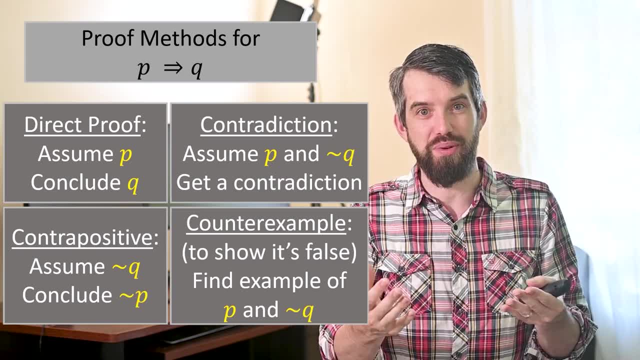 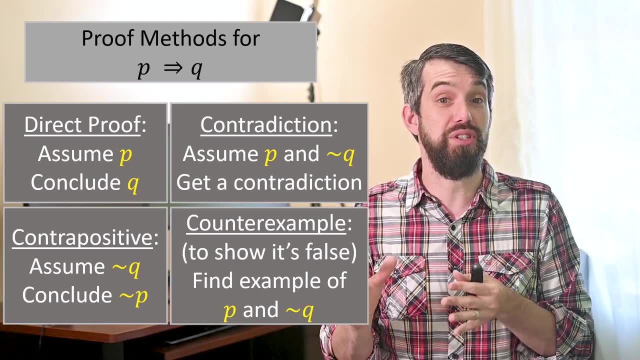 it's true in one example, but not show it is true in all examples. So that's a very important distinction. Now, to be fair, you might not know which of these methods you need to begin with until you really understand what proof is asking. but we're just showing at this stage what the 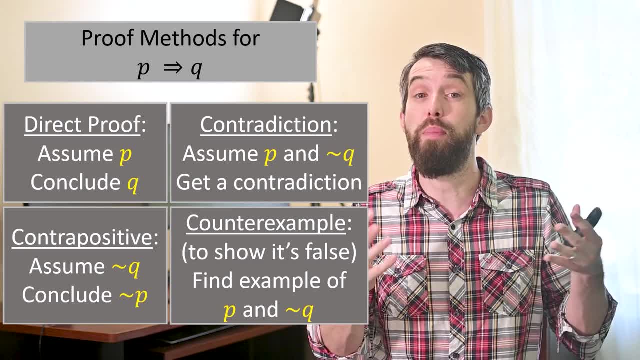 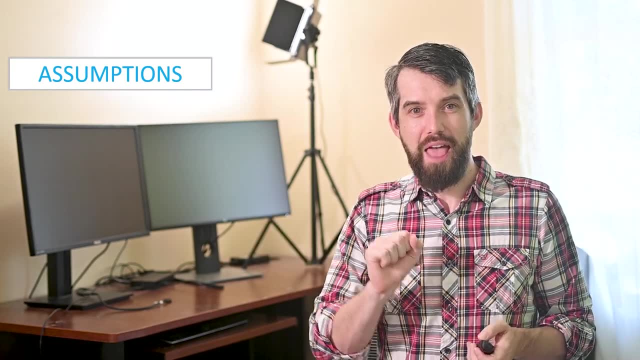 until you really understand what proof is asking. But we're just showing at this stage what the possibilities might be. Now, the reason I really like this is because the way I think about proofs is: I start with some assumptions and then I continue doing manipulations. 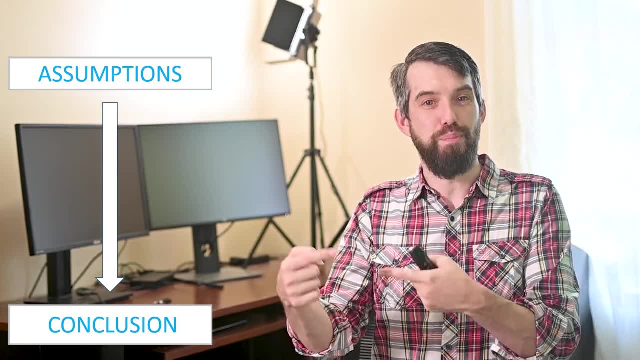 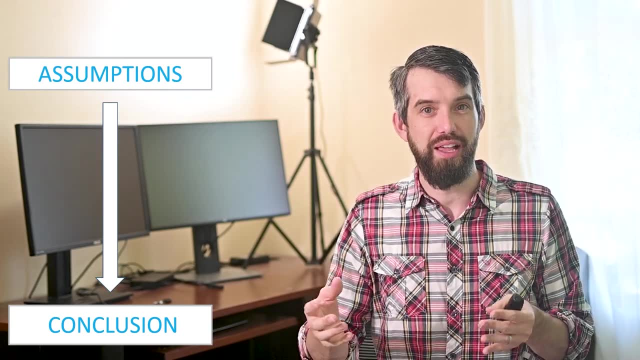 until I get to my conclusion, And what those different proof methods does is. it tells you what should you put in for the assumption and what should you put in for the conclusion. If you're doing a direct proof or a counter-proof or a positive, the assumption and the conclusion might differ. 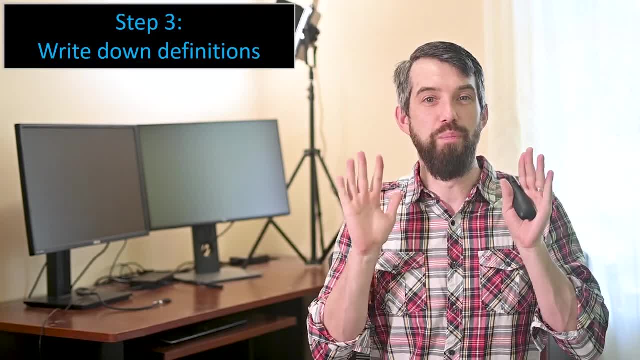 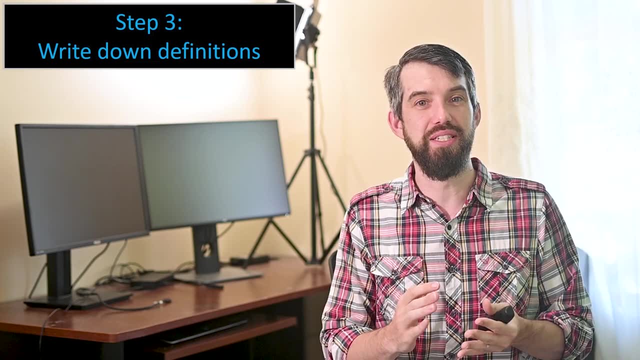 The next strategy might seem obvious, but it's actually super important and, for people who are at the beginning of their proof journey, a very easy one to miss. And that's just write down the definitions of every word in your assumptions and in your conclusions. 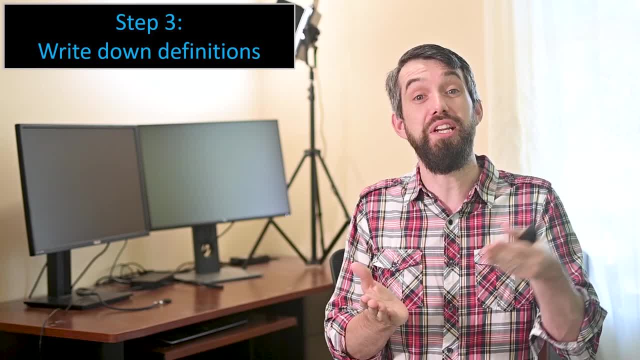 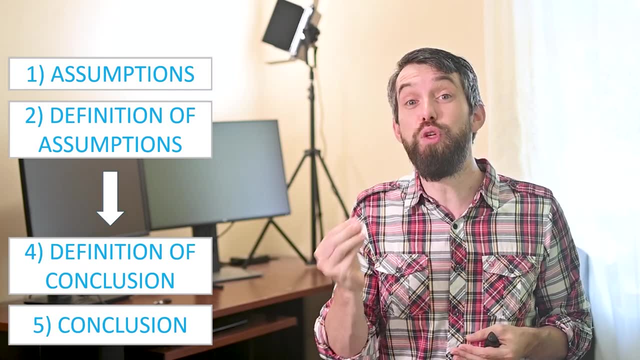 This is going to give you your first trick to being able to proceed in your proof. So remember we were just talking about how you might have assumptions and conclusions. Well, write down the definition of the words in the assumptions and write down the definition of the words. 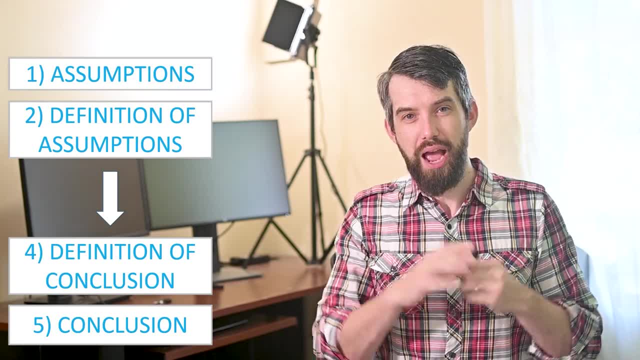 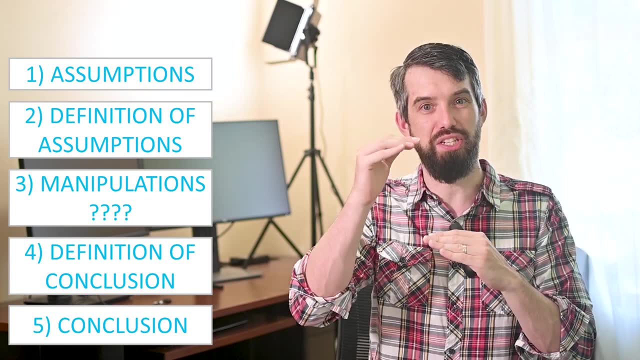 in the conclusions, their mathematical precise definition. And then what is in the middle? Well, the middle, what I call the step 3 here, is just the manipulations, all the ways that you can connect the top to the bottom. 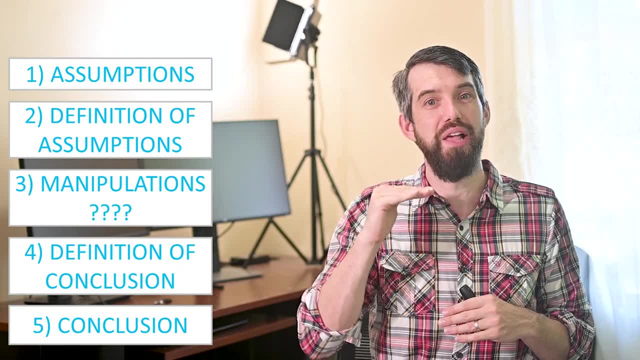 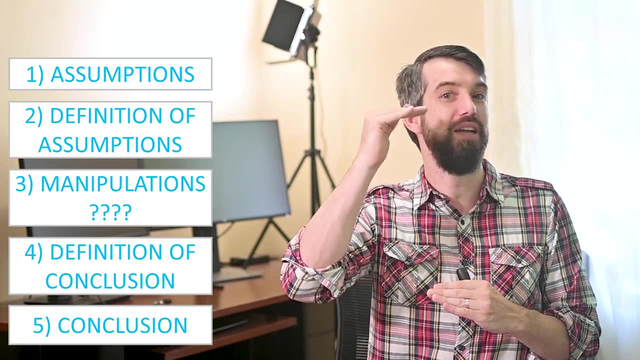 all the ways that you can go from your definition of your assumption down to the definition of your conclusion. That's sort of the hard part. But by scaffolding it this way with assumption, conclusion, definition of assumption and definition of conclusion, it will hopefully sort of make the gap between. 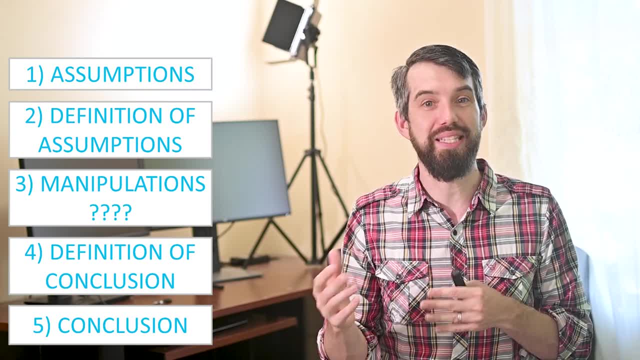 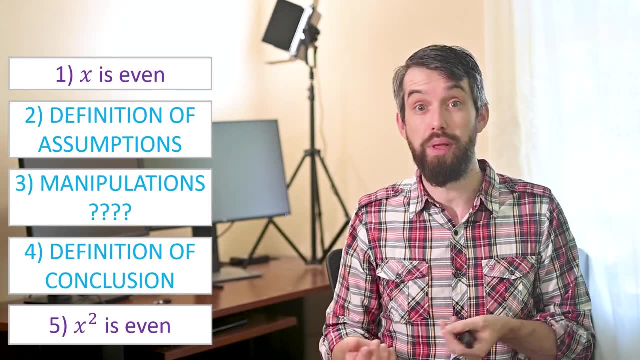 these where you have to do your manipulations smaller. Okay, so let's see an example. in the case where we had- if x was even, then x squared was even, I can write down my assumption and my conclusion. So my assumption is that: 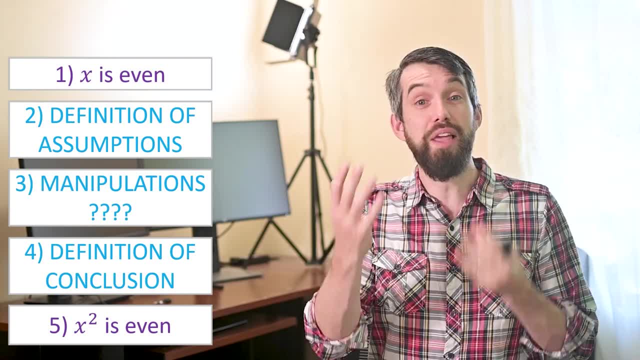 x is even and my conclusion is that well, x squared is even. So I just write those down at the beginning and the end of my proof, And the next thing I have to do is: what do I mean by even? What is the definition of that? 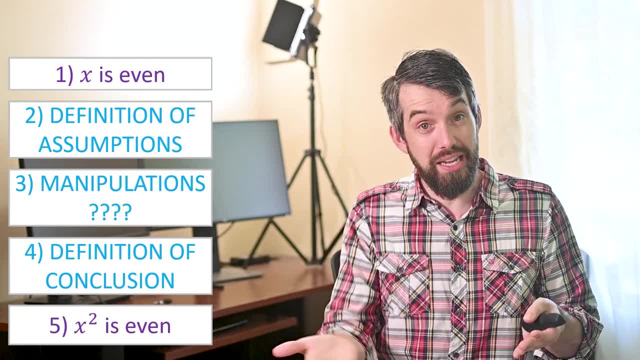 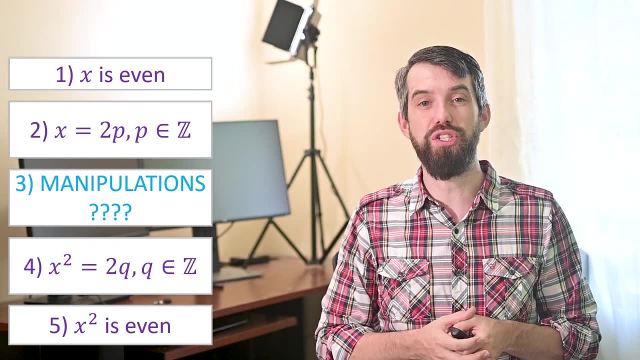 And even has a very precise definition. It means it's twice an integer, So, for example, 6 is twice 3, and 8 is twice 4, and so forth. So I can write down what my definitions are. My definition is that x is 2p. 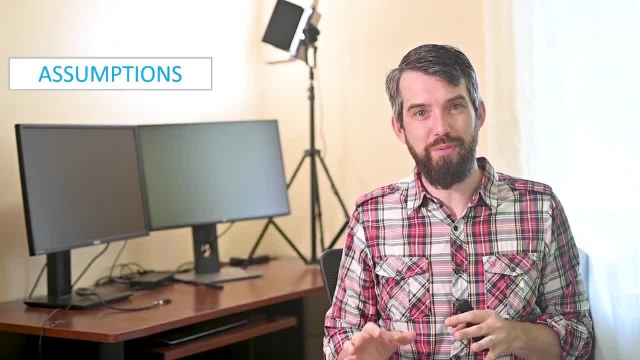 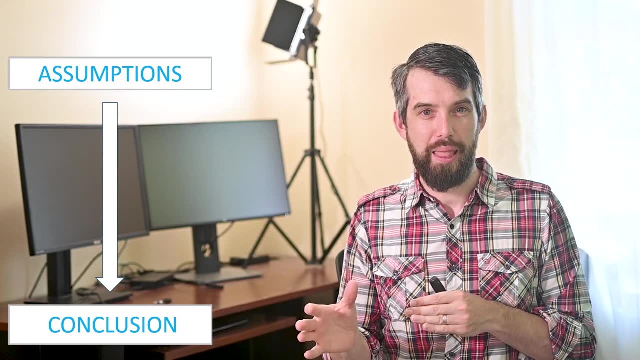 possibilities might be. Now, the reason I really like this is because the way I think about proofs is: I start with some assumptions and then I continue doing manipulations until I get to my conclusion. And what those different proof methods does is: it tells you what should you. 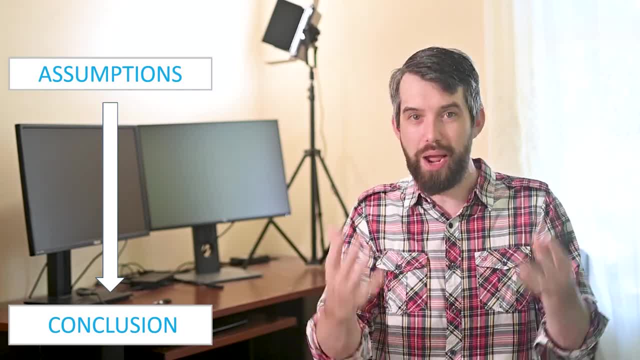 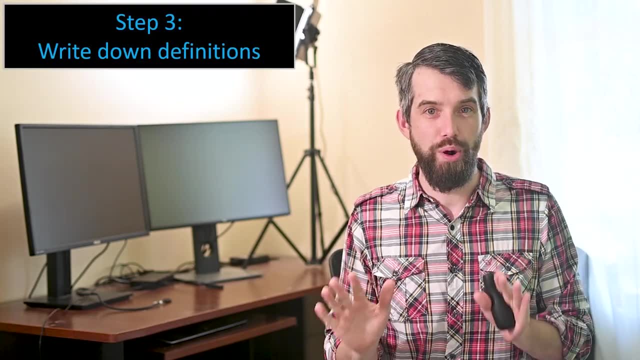 put in for the assumption and what should you put in for the conclusion? If you're doing a direct proof or counterpositive, the assumption and the conclusion might differ. The next method might seem obvious, but it's actually super important and for people who are at the 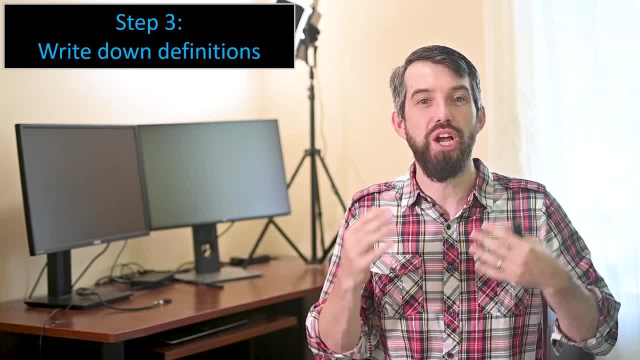 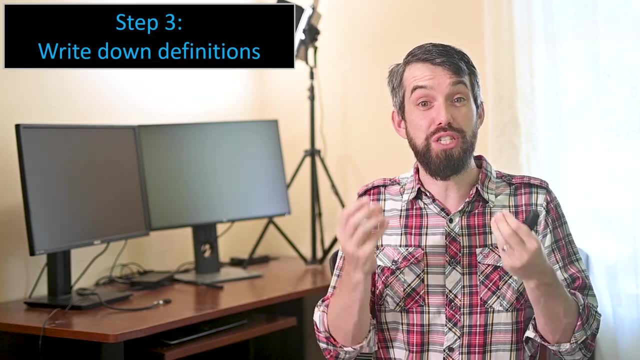 beginning of their proof journey- a very easy one to miss- and that's just write down the definitions of every word in your assumptions and in your conclusions. This is going to give you your first trick to being able to proceed in your proof. So remember, we were just talking about how you might. 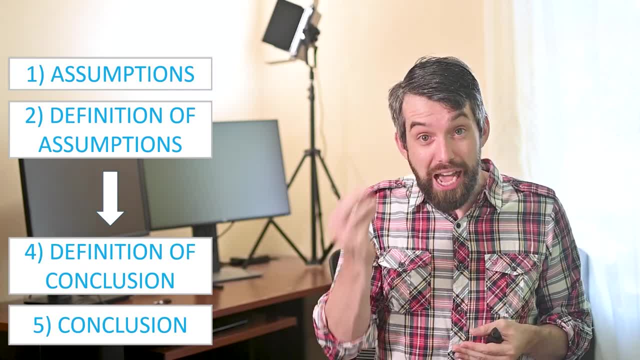 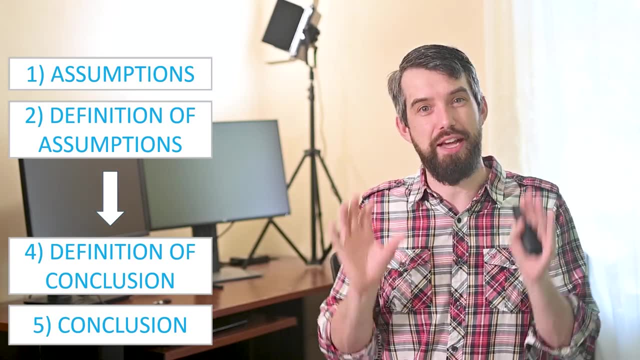 have assumptions and conclusions. Well, write down the definition of the words in the assumptions and write down the definition of the words in the conclusions. They're mathematical, precise definitions. And then, what is in the middle? Well, the middle, what I call the step three here. 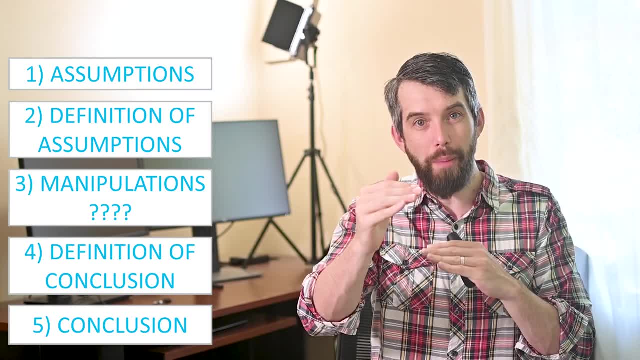 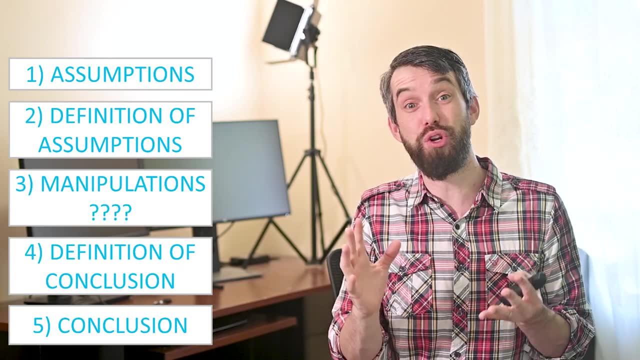 is just the manipulations, All the ways that you can connect the top to the bottom, All the ways that you can go from your definition of your assumption down to the definition of your conclusion. That's sort of the hard part, but by scaffolding it this way with assumption, 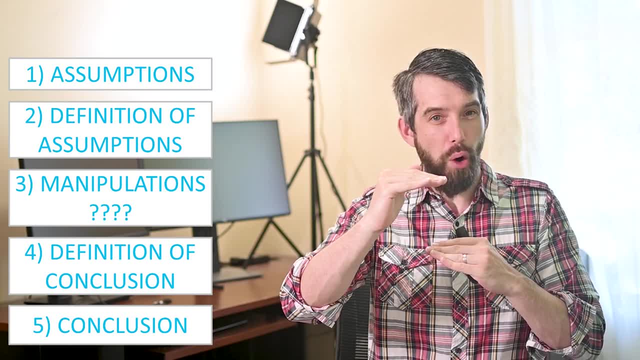 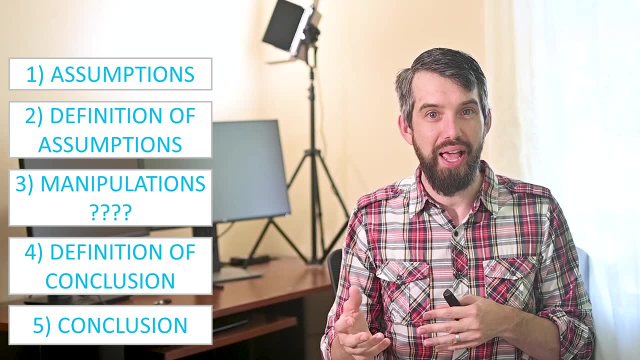 conclusion: definition of assumption and definition of conclusion. it will hopefully sort of make the gap between these, where you have to do your manipulations, a bit smaller. Okay, so let's see an example. So let's say, for example, in the case where we had, if x was even, then x squared was even, I can write: 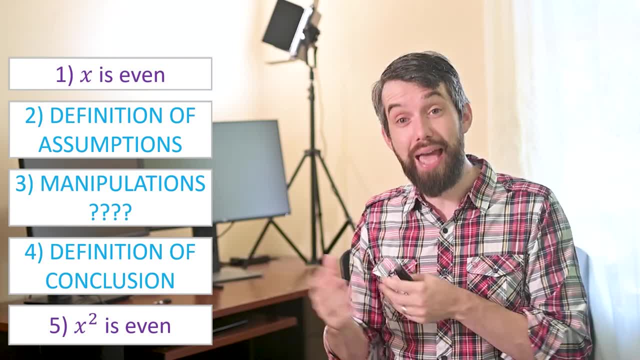 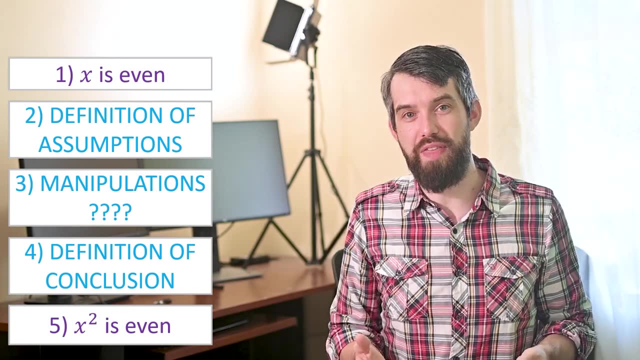 down my assumption and my conclusion. So my assumption is that x is even and my conclusion is that, well, x, squared, is even. So I just write those down at the beginning and the end of my proof And the next thing I have to do is: what do I mean by even? What is the definition of that? 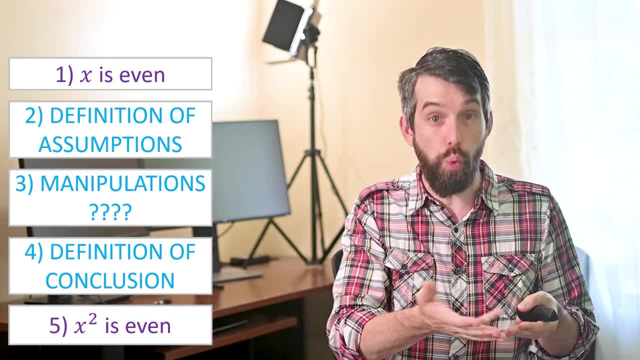 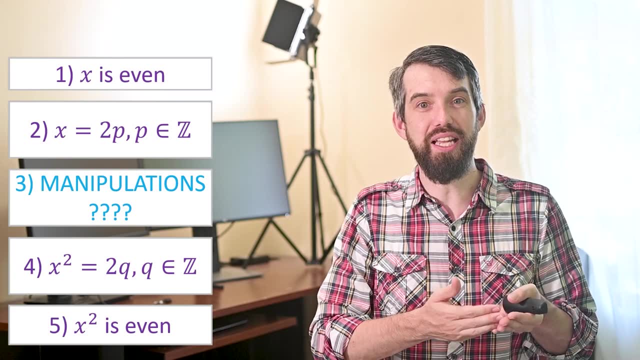 An even has a very precise definition. It means it's twice an integer. So, for example, six is twice three and eight is twice four and so forth are. My definition is that x is 2p where p is an integer, and my definition of my conclusion. 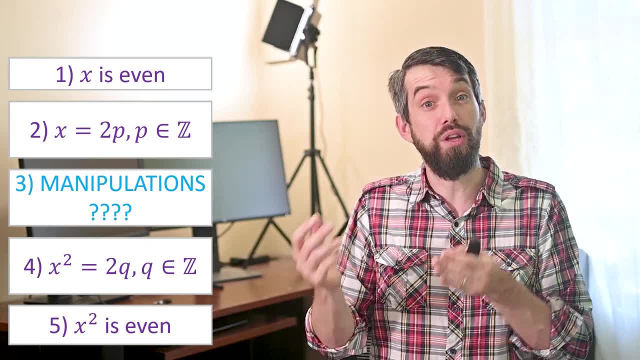 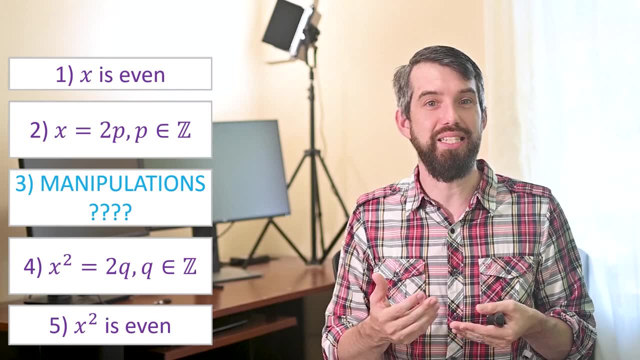 which is that x squared is even, is that x squared is equal to 2q, where q is an integer. One of the things that happens in this stage is you often want to introduce variable names. I mean, in both cases of the assumption and the conclusion, I'm introducing an integer. 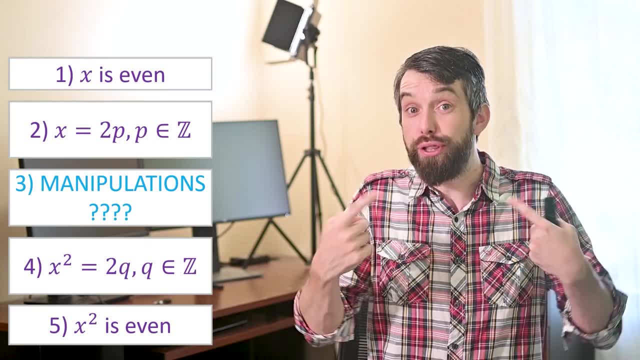 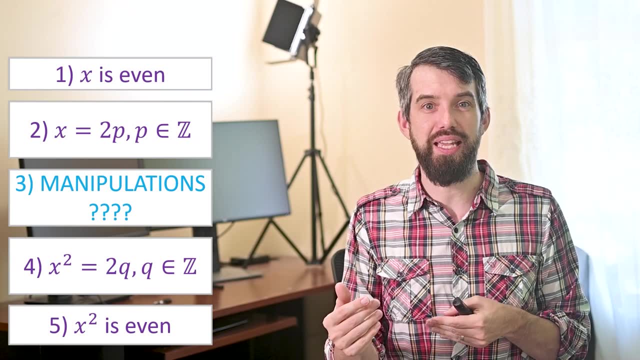 where p is an integer, and my definition of my conclusion, which is that x squared is even, is that x squared is equal to 2q where q is an integer. One of the things that happens in this stage is you often want to introduce variable names. 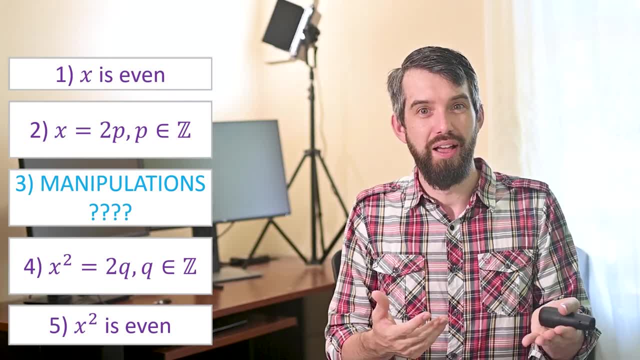 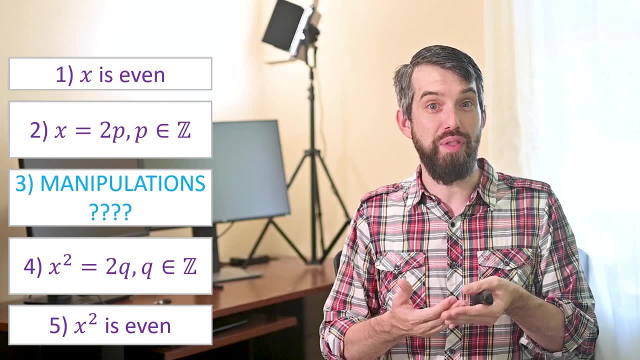 I mean in both cases of the assumption and the conclusion. I'm introducing an integer, but I don't want to repeat myself because they're representing both x or x squared respectively. So I use p for the x and q for the x squared. 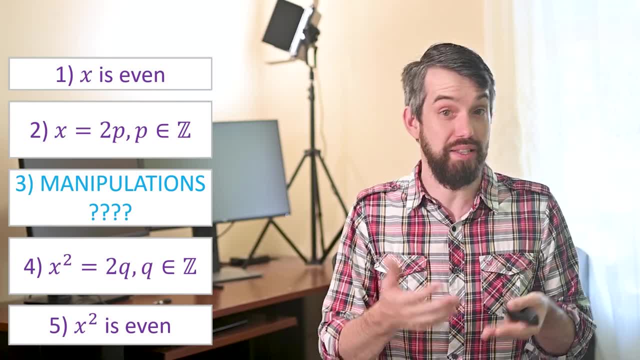 And part of your proof will involve defining some notation like this. In this case, I'm defining: where the p lives, it's an integer, and where the q lives, it's also an integer. Okay, so now we have the manipulations. 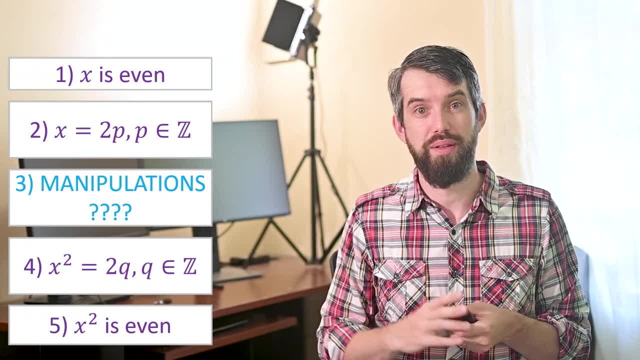 And that again is the hard part. but I mean, if you want to, you could. But now we have manipulations And, if you wish, you can always pause the video and try to see it before I'm going to spoil it for you. 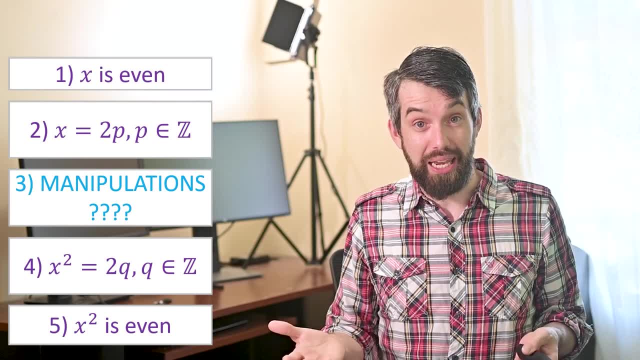 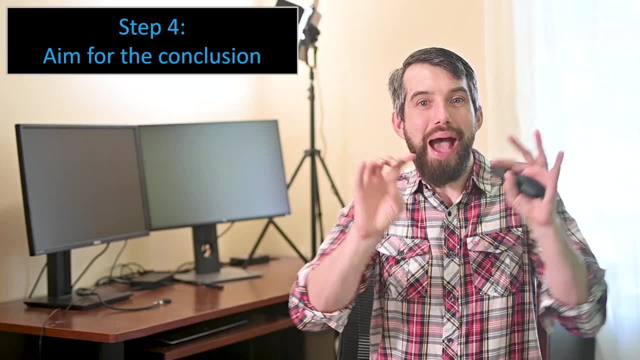 Okay, next step. I want to try to figure out those manipulations. but how do I do this? Well, I really want to have a goal of going towards. whatever that conclusion is, I know I'm at the assumption. That's my sort of starting spot. 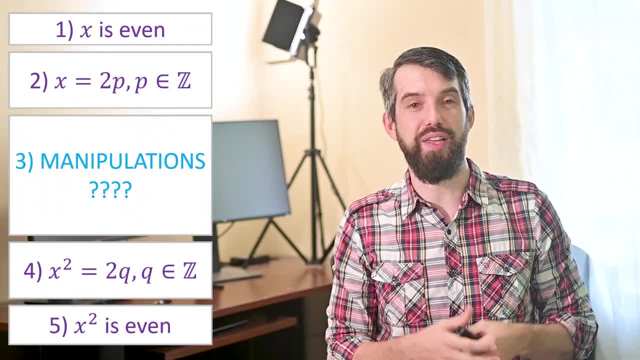 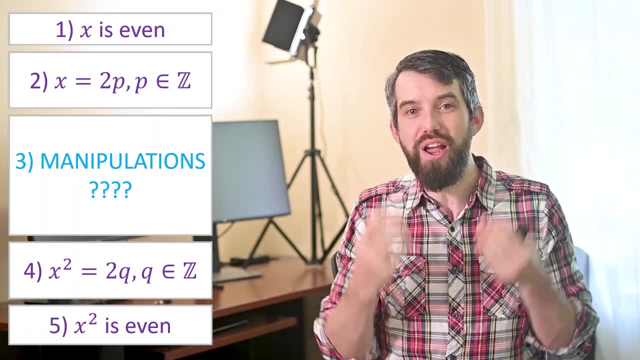 And I want to head in the direction of the conclusion. So what we were just looking at with this x even implies x squared. even Because the conclusion has something to do with x squared, there's really a very natural manipulation to do. I have an x. 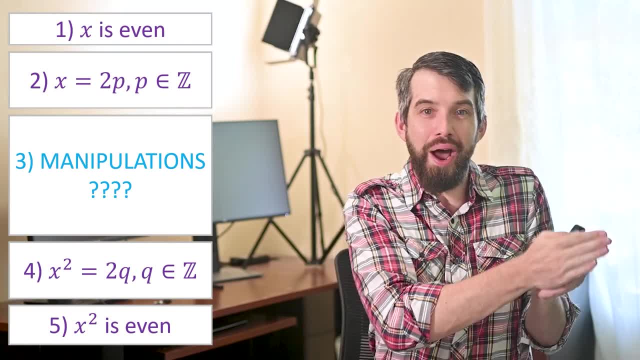 I want to get to an x squared. So if I'm looking at the conclusion and trying to make what I have look like what I want, the natural thing to do is to square my x, And so that's what I do for manipulation. 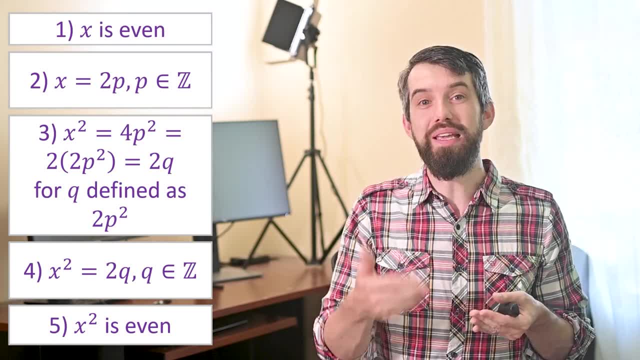 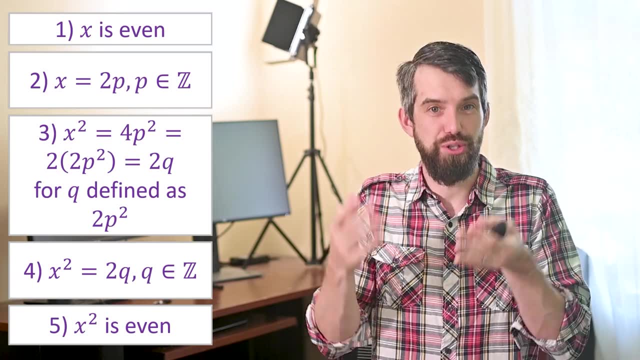 I square it And I notice that this is going to give me 4p squared, And since I want to write that x squared as twice something, so I just factor a 2 out and write this as 2 times 2p squared. 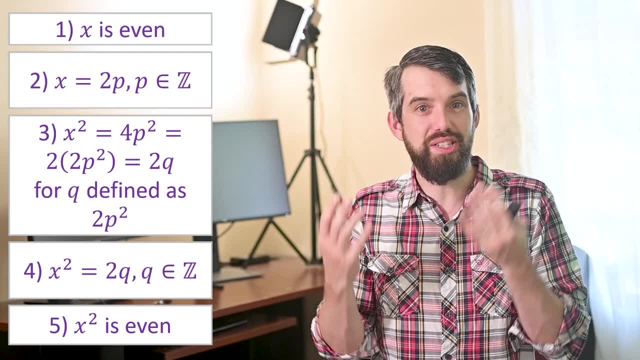 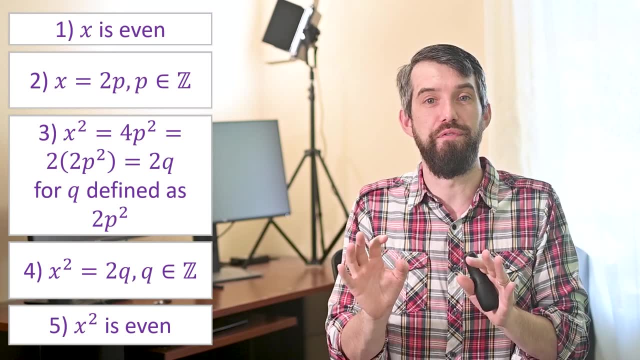 And then that's exactly of the form 2 times something, where that something is this 2p squared, And I'll just call that q. So define my q and that is my proof. This is a complete proof of this particular claim. 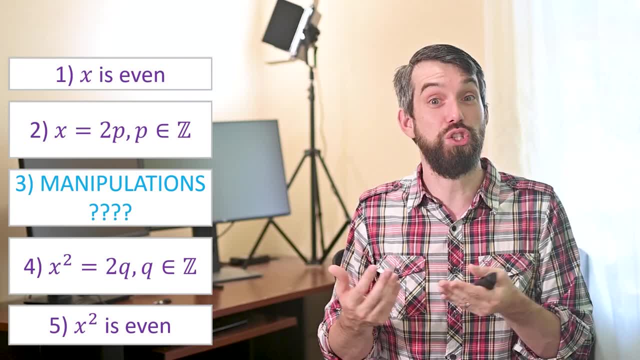 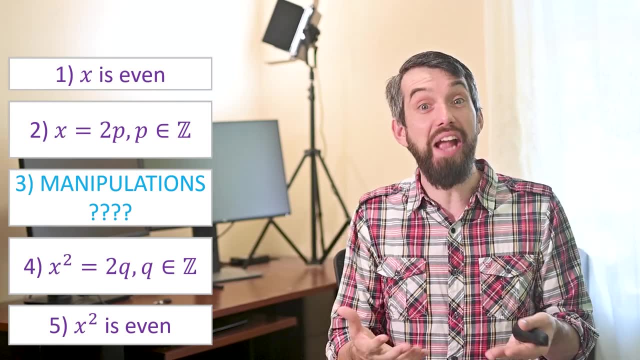 but I don't want to repeat myself, because they're representing both x or x squared respectively. so I use p for the x and q for the x squared. So part of your proof will involve defining some notation like this. In this case I'm defining where the p lives- it's an integer- and where 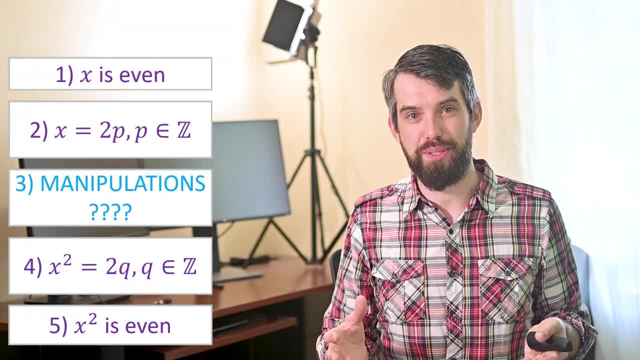 the q lives, it's also an integer Okay. so now we have the manipulations, and that again is the hard part. but I mean, if you want to, you could. but now we have manipulations and if you wish, 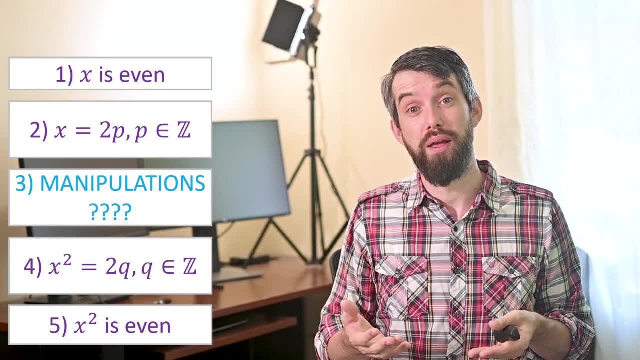 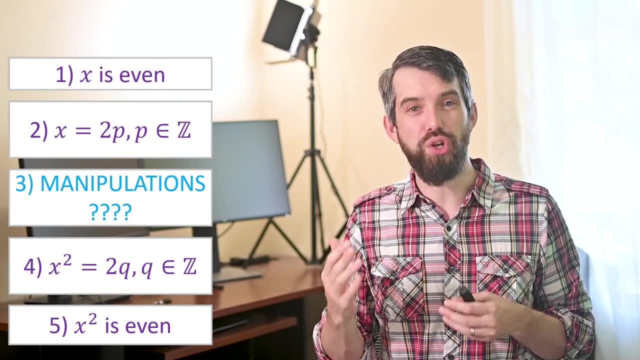 you can always pause the video and try to see it before I'm going to spoil it for you. Okay, next step. I want to try to figure out those manipulations. but how do I do this? Well, I really want to have a goal of going towards. whatever that conclusion is, I know I'm at the 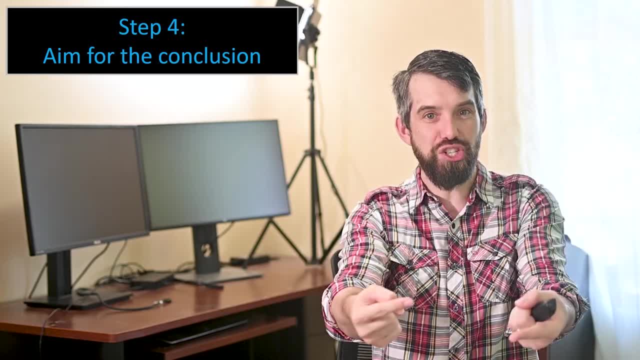 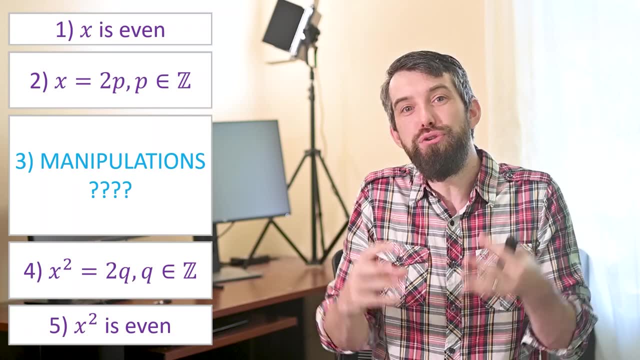 assumption. that's my sort of starting spot and I want to head in the direction of the conclusion. So what we were just looking at with this x even implies x squared, even because the conclusion has something to do with x squared. there's really a very natural. 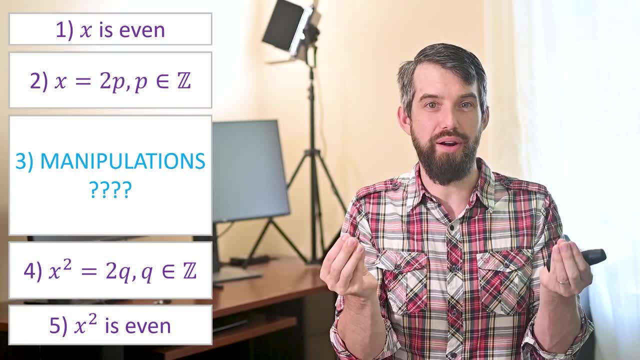 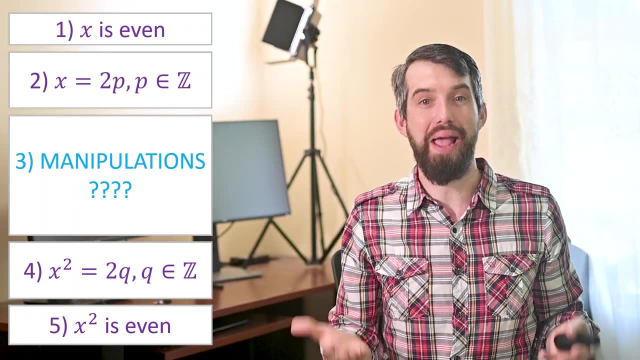 manipulation to do. I have an x. I want to get to an x squared. so if I'm looking at the conclusion and trying to make what I have look like what I want, the natural thing to do is to square my x, And so that's what I do for manipulation: I square it and I notice that this is going to give me. 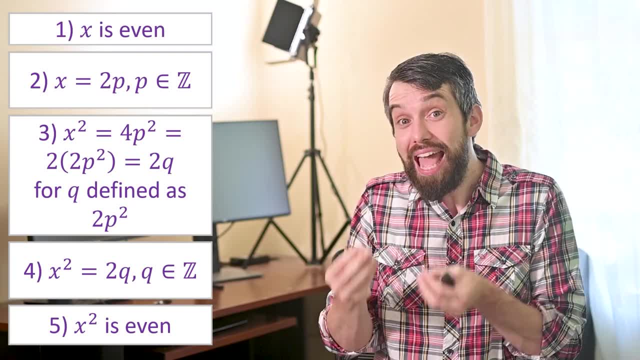 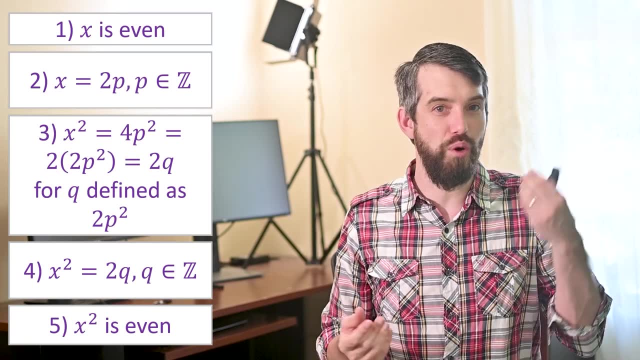 four p squared. and since I want to write that x squared as twice something, so I just factor a two out and write this as two times two p squared, and then that's exactly of the form two times something, where that something is this: two p squared, and I'll just call that q. So define my. 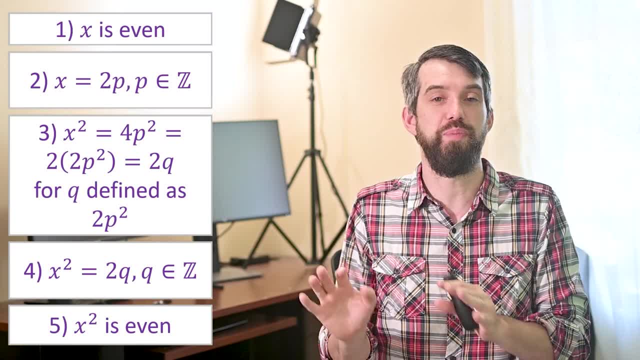 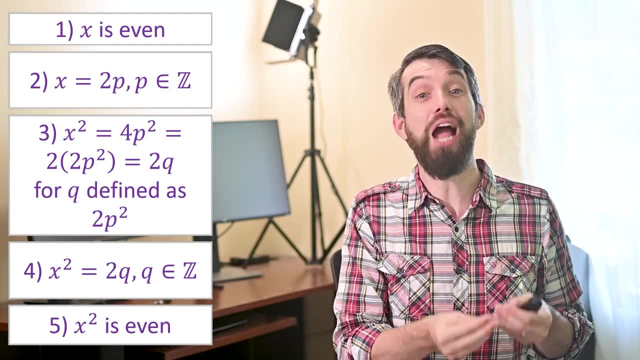 q, and that is my proof. This is a complete proof of this particular claim. So the point here was that I found a direction for what my goal was, and I found a direction for what my goal was and I found a direction for what manipulations I should do by saying I want my assumptions to look. 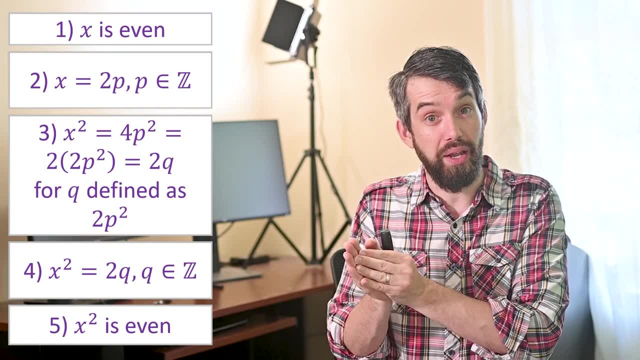 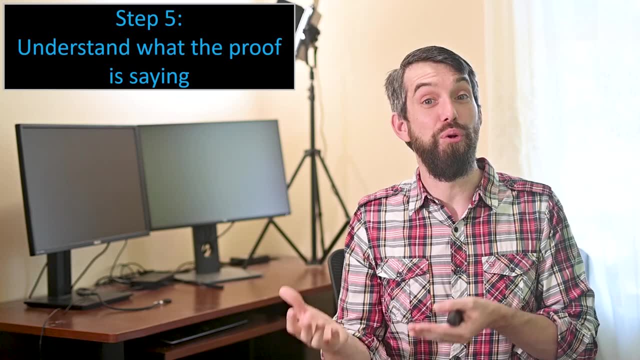 like the conclusions, but I had to square it and write it as twice something, and that gave me all the ideas that I needed for my manipulations. So that was some of the scaffolding, the sort of logical structures that I like to think about when coming up with my proof, And now we actually have. 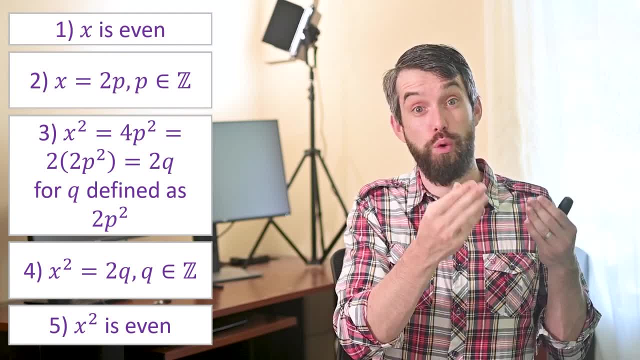 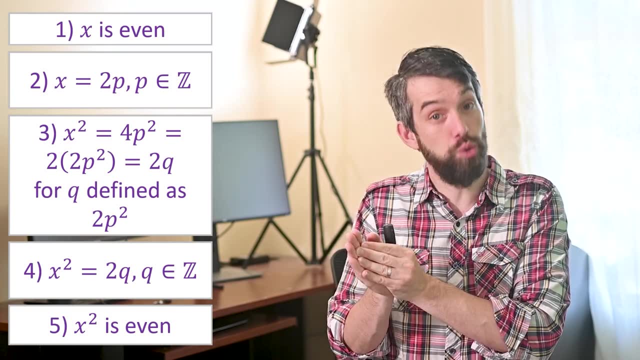 So the point here was that I found a direction for what manipulations I should do by saying I want my assumptions to look like the conclusions, but I had to square it and write it as twice something, And that gave me all the ideas that I needed. 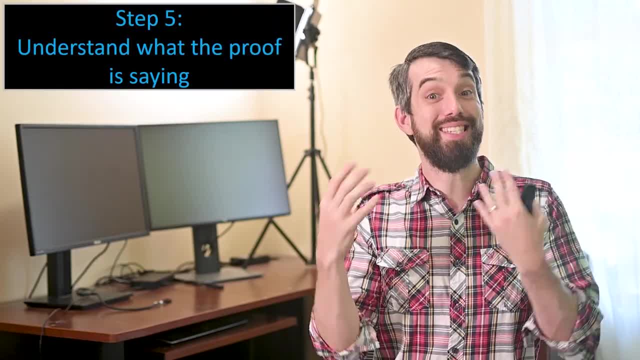 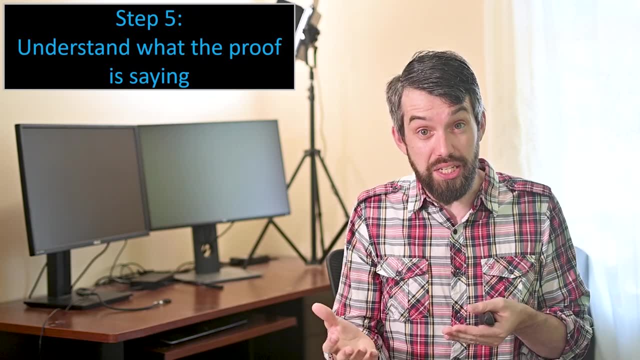 for my manipulations. So that was some of the scaffolding, the sort of logical structures that I like to think about when coming up with my proof. And now we actually have to proceed to something. We actually have to proceed to those manipulations. 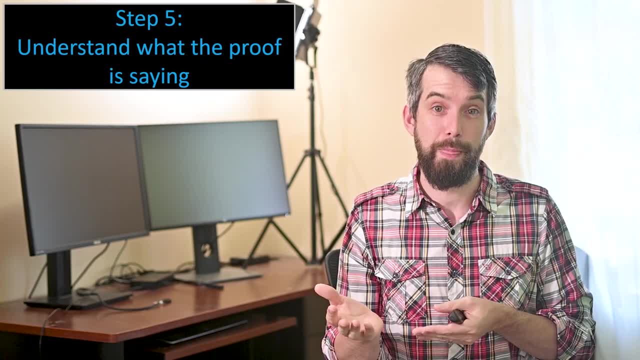 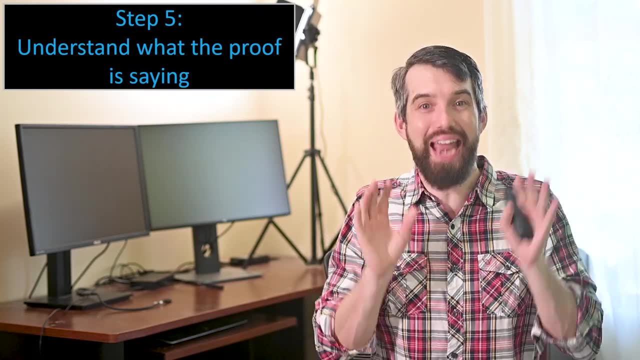 And maybe even if you aim for manipulations, you don't see a path forward, And in fact everything that you've done previously could almost be done without having any idea about what the statement meant at all, which is sort of a bit bizarre. 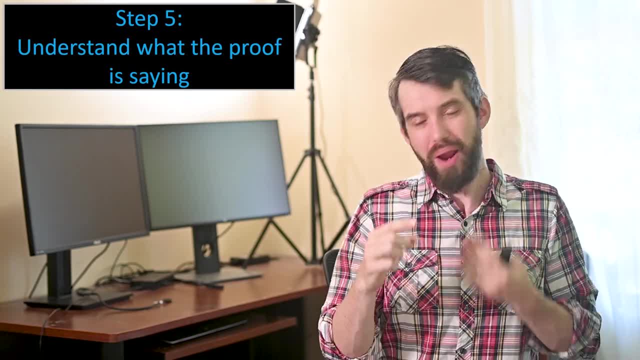 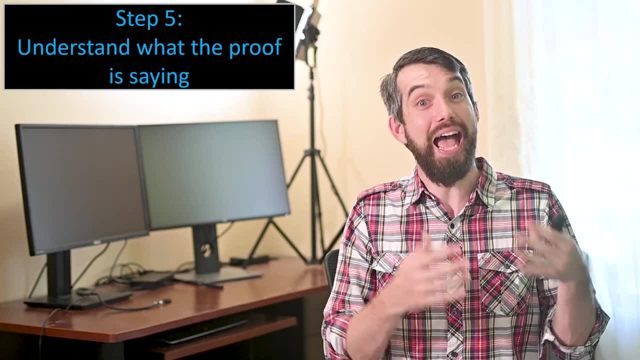 Perhaps you want to try to understand the statement first. Maybe that should be step one, But I put it down here because this is when it really transitions to not just following this cookie-cutter method that I've outlined, but to actually using your own. 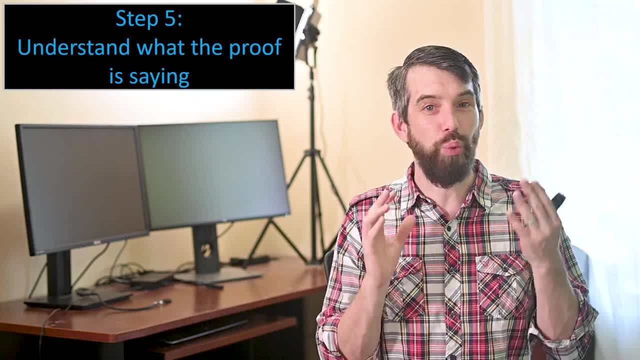 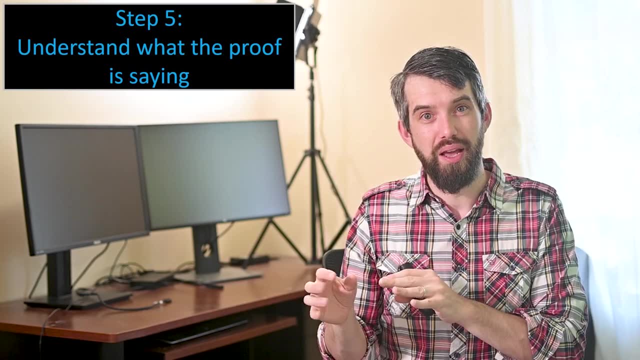 intuition, your own understanding. So I really try to read the statement and try to understand. what is it asking? What does the assumption mean? What does it mathematically mean? What does the conclusion mean? What does this connection sort of feel like? 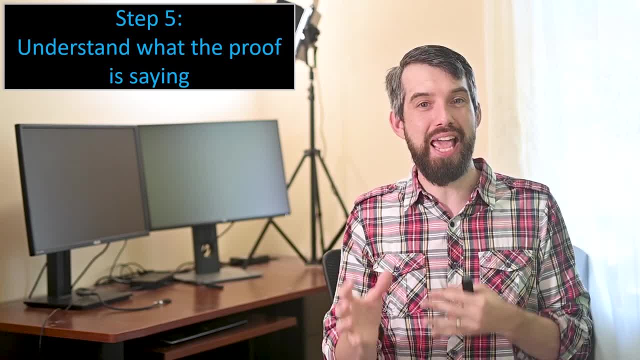 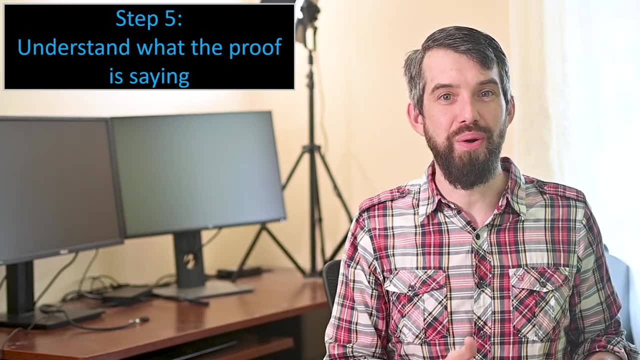 what does it look like? I try to really have a nice sort of large-scale understanding of what this is actually asking before I try to actually go and prove it. The next thing I really like to do is to well is just basically draw a picture. 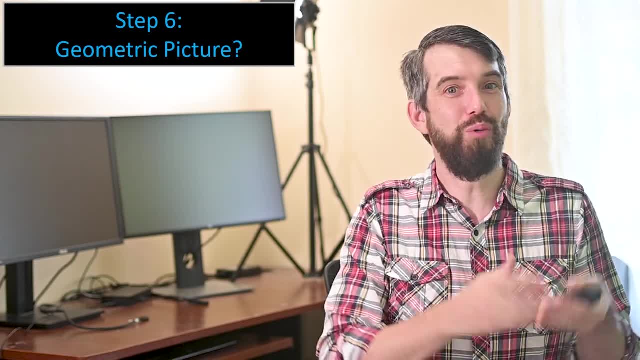 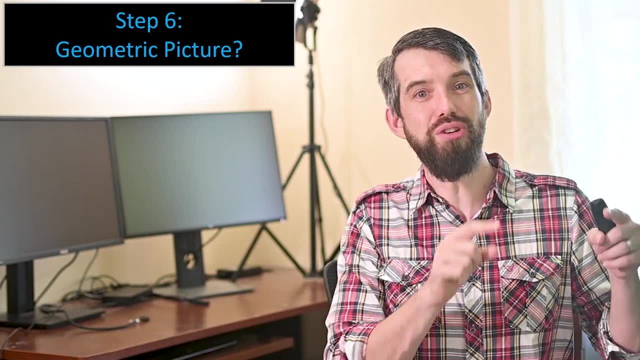 It depends on what type of proof it's going to be. This business with the x-squares, well, there wasn't really a nice natural geometric picture, For example linear algebra. there's all kinds of beautiful pictures that you want to draw. So does your statement. 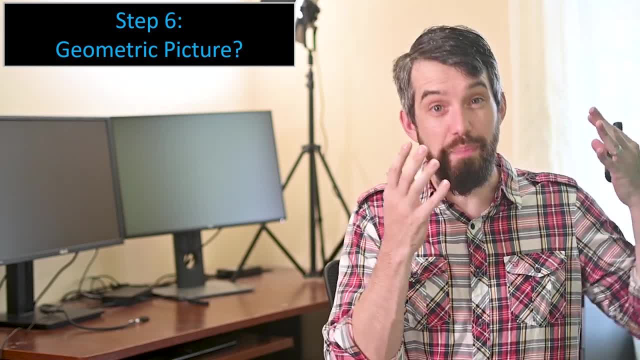 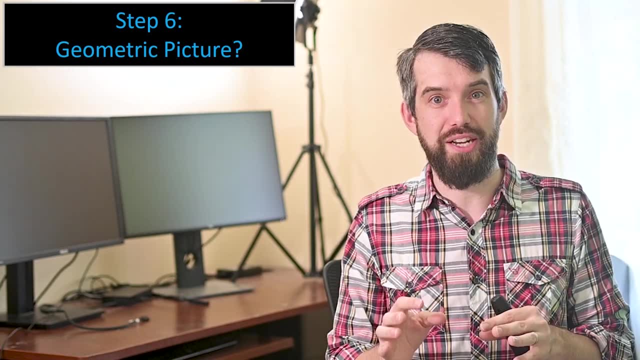 that you're trying to prove. could you represent it geometrically? Is there a picture that interprets the assumptions or interprets the conclusion and tries to see how those might be connected? If you can draw a picture, a lot of the time mathematics is just writing down the picture. 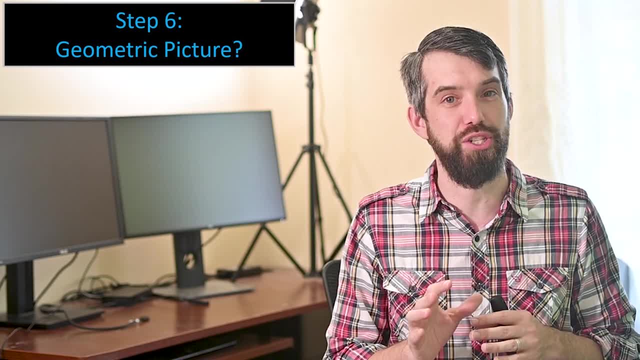 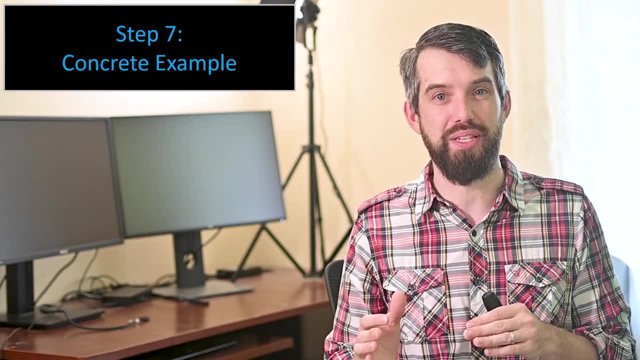 that you're able to draw, So I'd really encourage you to try to come up with a beautiful geometric picture, if you can. The next thing I really like to do is to come up with some specific examples. I mean, I already talked about 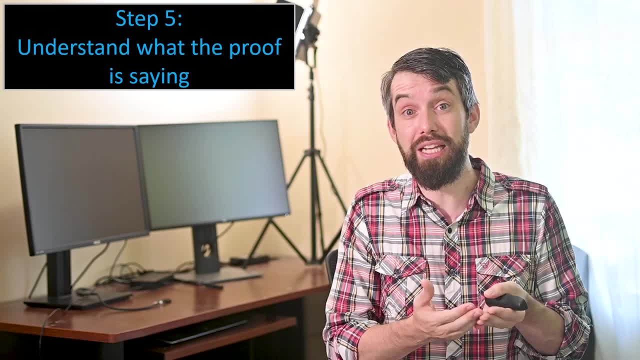 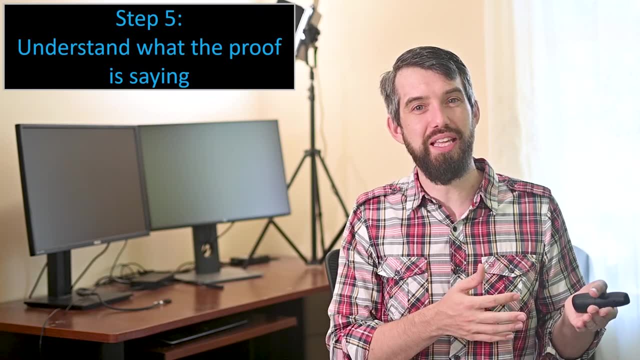 to proceed to something We actually have to proceed to those manipulations, and maybe even if you aim for manipulations, you don't see a path forward, And in fact, everything that you've done previously could almost be done without having any idea about what the statement meant at all. 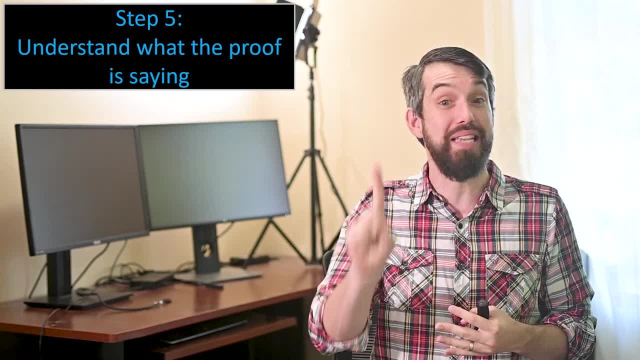 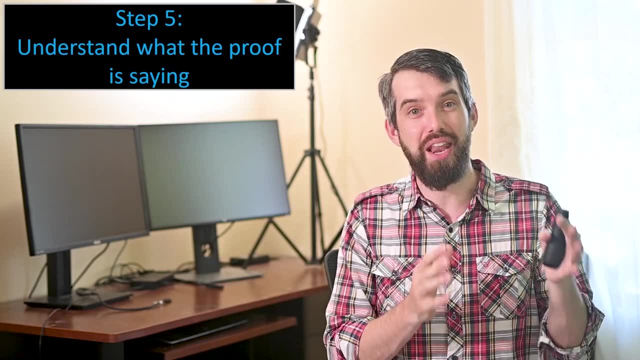 which is sort of a bit bizarre. Perhaps you want to try to understand the statement first. Maybe that should be step one, But I'm putting it down here because this is when it really transitions to not just following this cookie cutter method that I've outlined, but actually using your own. 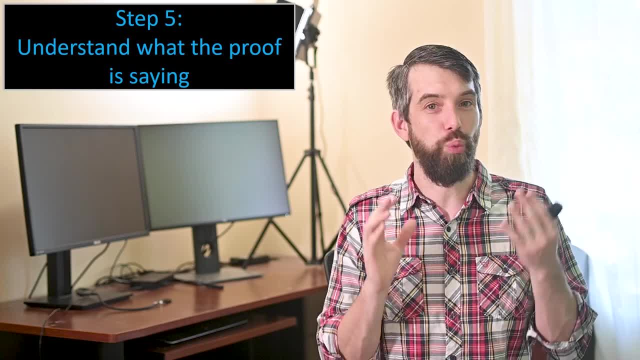 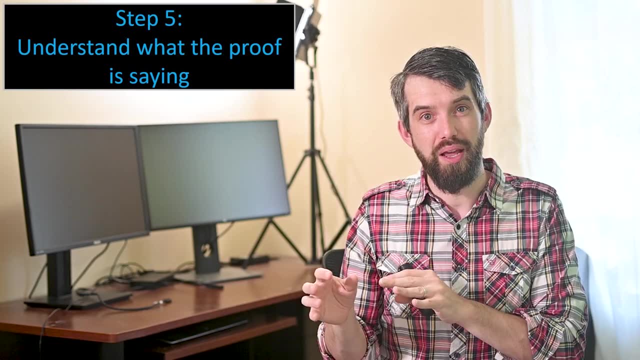 intuition, your own understanding. So I really try to read the statement and try to understand. what is it asking? What does the assumption mean? What does it mathematically mean? What does the conclusion mean? What does this connection mean? What does the conclusion mean? What does this? 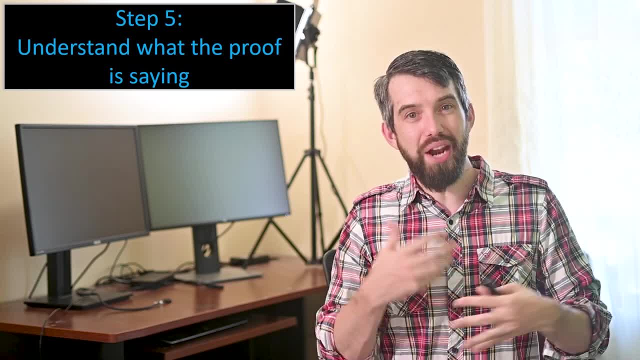 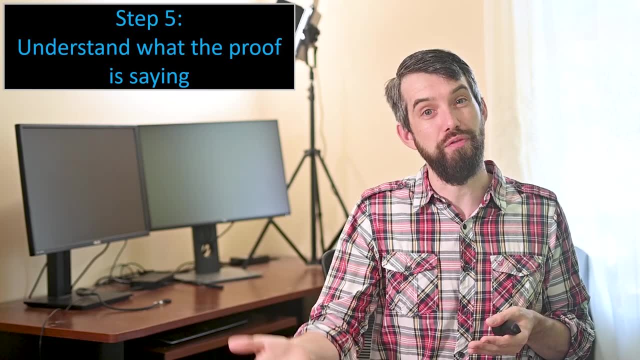 connection, sort of feel like or look like. I try to really have a nice sort of large scale understanding of what this is actually asking before I try to actually go and prove it. The next thing I really like to do is to- well, it's just basically draw a picture. It depends on. 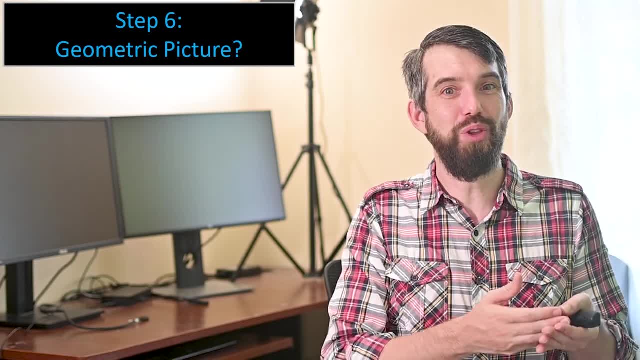 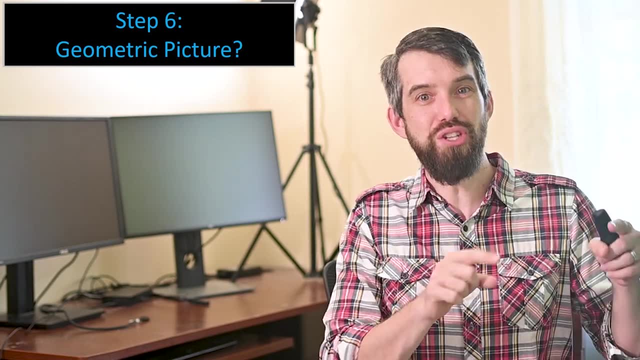 what type of proof it's going to be This business with the x squareds? well, there wasn't really a nice natural geometric picture. For example, in linear algebra there's all kinds of beautiful pictures that you want to draw, So does your statement that you're trying to prove, could you? 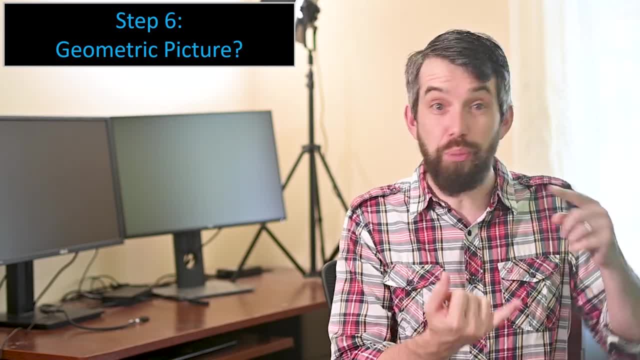 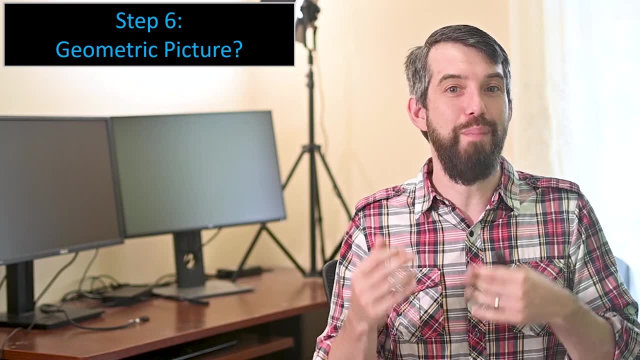 represent it geometrically. Could you draw a picture that interprets the assumptions or interprets the conclusion and tries to see how those might be connected? If you can draw a picture, a lot of the time mathematics is just writing down the picture that you're able to draw. 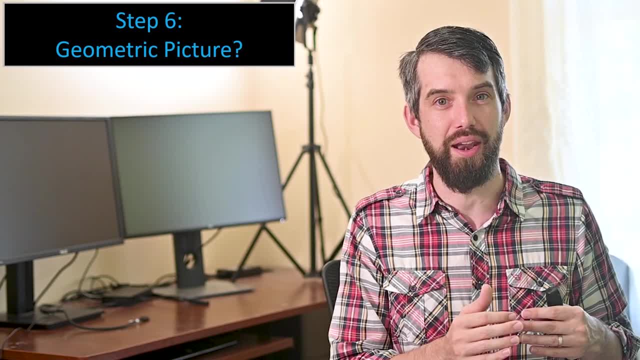 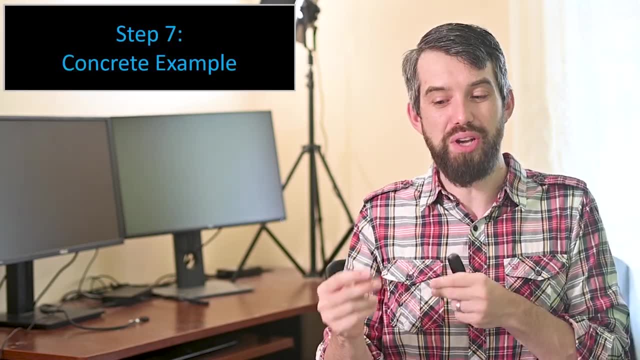 So I'd really encourage you to try to come up with a beautiful geometric picture, if you can. The next thing I really like to do is to come up with some specific examples. I mean, I already talked about how you cannot use a concrete example as your proof, But that doesn't mean concrete. 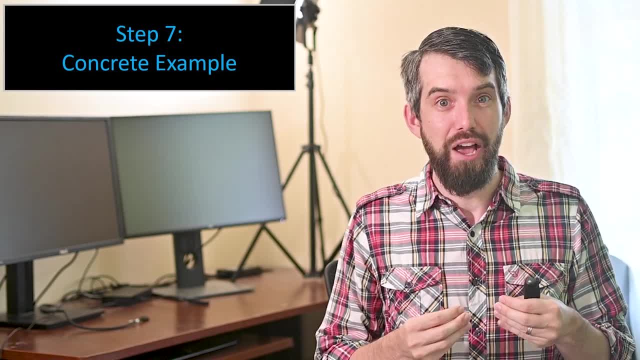 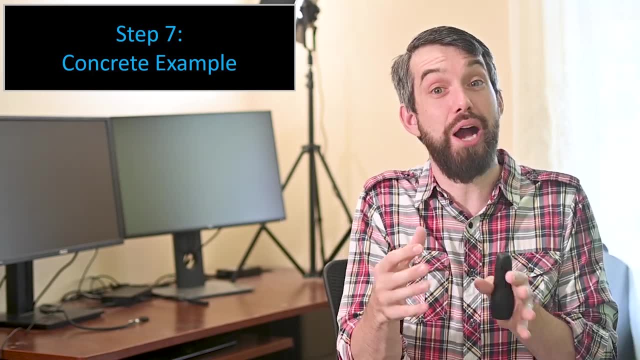 examples. Indeed, a concrete example is extremely valuable for giving you intuition. So I would put in some numbers, I would choose a specific instance and I would try and compute it out in that specific instance and see why might the conclusion be connected to the assumption. Can 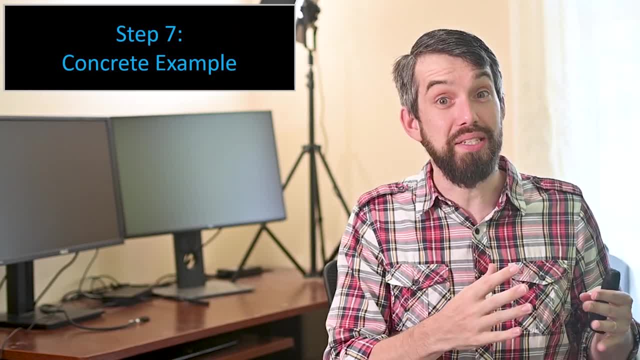 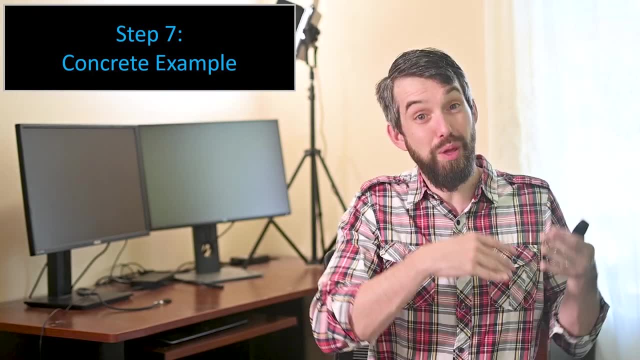 I understand that in one concrete example, If I can do it once, I might be able to then generalize and prove it arbitrarily Indeed. this sort of connects to the point of drawing a geometric picture. Maybe you want to draw the geometric picture in a specific example. 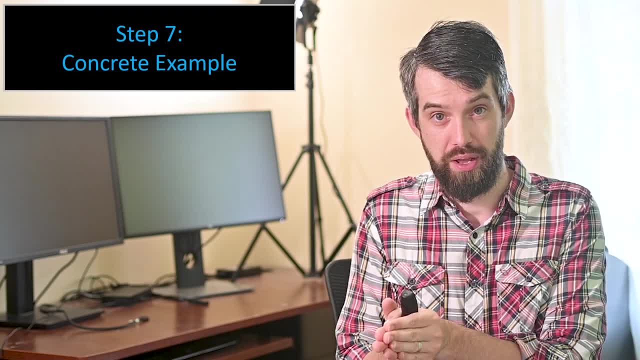 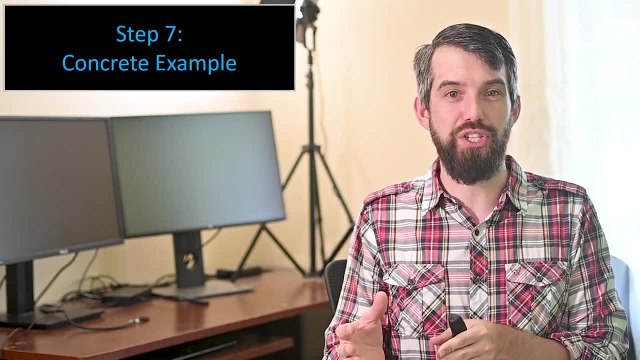 how you cannot use a concrete example as your proof, But that doesn't mean concrete examples are pointless. Indeed, a concrete example is extremely valuable for giving you intuition, So I would put in some numbers, I would choose a specific instance and I would try and compute it out. 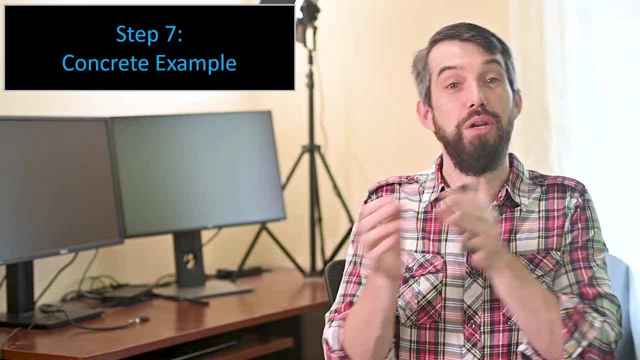 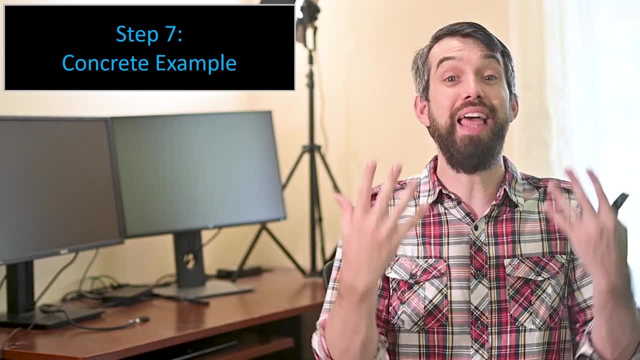 in that specific instance And see why might the conclusion be connected to the assumption? Can I understand that in one concrete example, If I can do it once, I might be able to then generalize and prove it arbitrarily Indeed? this sort of connects? 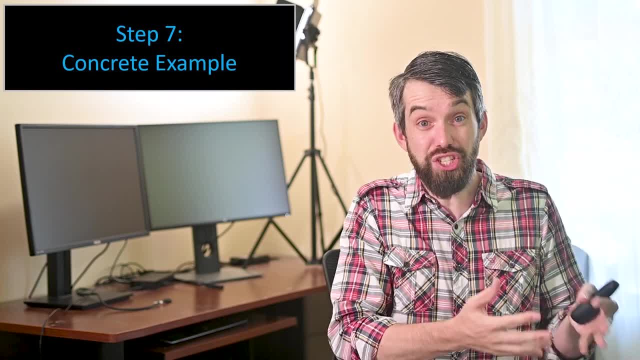 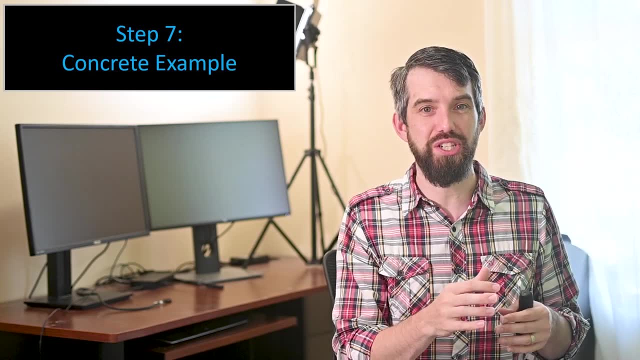 to the point of drawing a geometric picture. Maybe you want to draw the geometric picture in a specific example, something that you know about. Indeed, anytime I'm learning a new mathematics field, if there's some new definitions, I always try to write down. 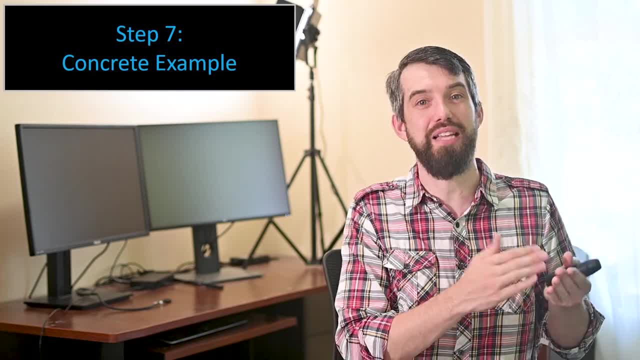 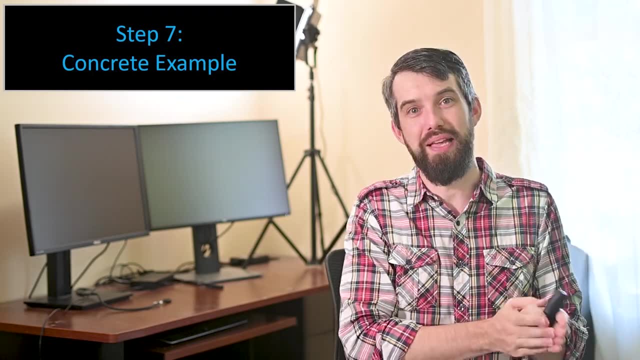 as many little examples as I can that explore a specific definition. Look at the idea of a basis. I just try to draw as many little examples of a basis until I understand what is a basis, what is not a basis. I feel that sort of doing. 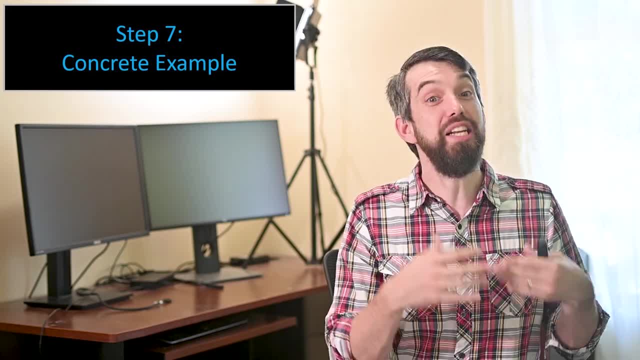 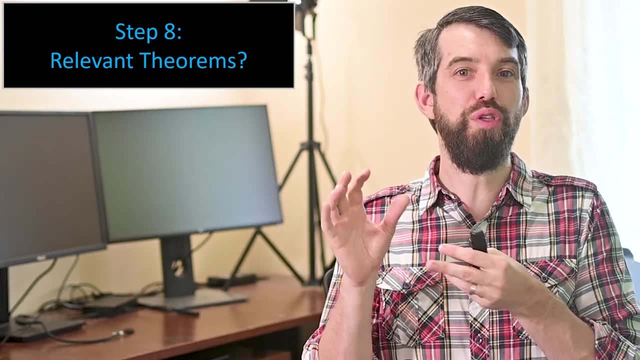 that exploring through canonical examples is an extremely important part of doing mathematics. The next thing I often look for if I'm not getting any ideas is: what are the relevant theorems about the kind of mathematical object that I'm talking about When I look? 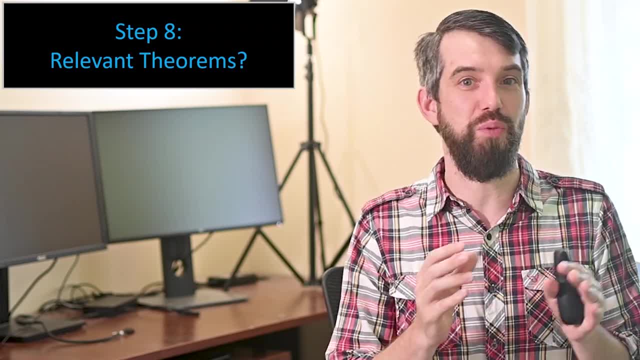 at the assumptions. when I look at the conclusions, I want to know what are the major theorems that we see. If you're in a course, you'll often get these from your textbook and it'll be taught about in class. These are the major. 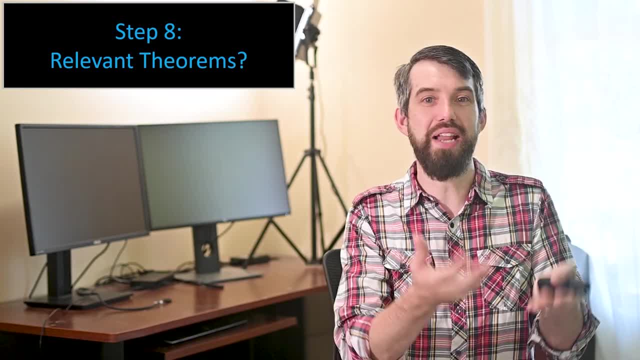 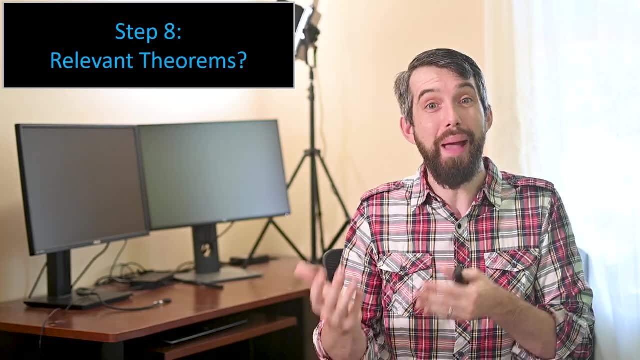 ideas that you need Indeed. a lot of proofs are basically just write down the definitions, see what theorems apply and sort of connect those together to get to the assumptions. That's sort of the core math. that's just linking one or two theorems to the definitions that you 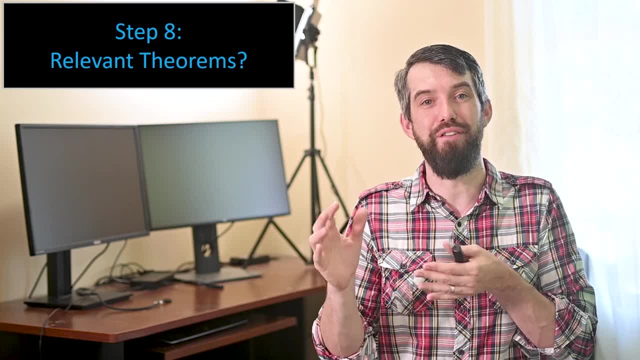 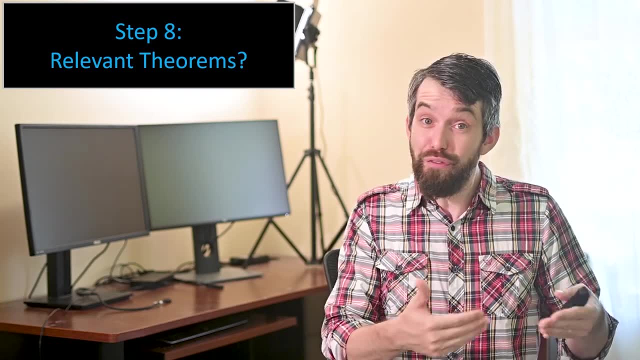 actually have. I really encourage you to sort of see what's available here, And, if you want to, you could even go a little bit further. This doesn't always work, but sometimes, if you read the proofs of the relevant theorems, then 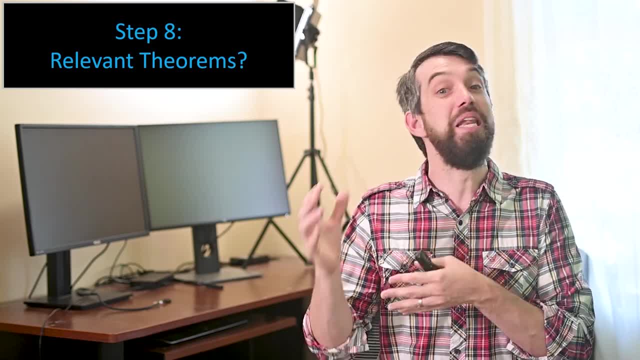 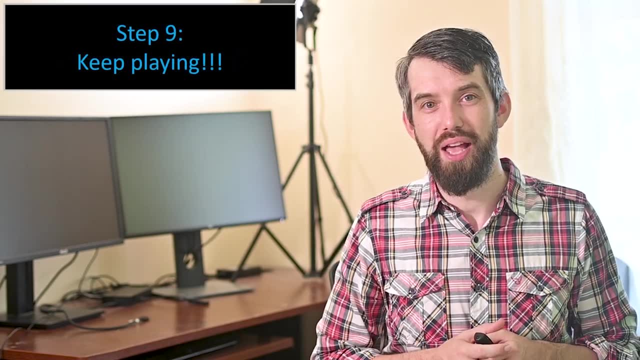 that can give you ideas for the types of manipulations people do with the objects that are in the theorem that you're talking about. And then the final thing I'm going to talk about is really just to sort of play around. I've noticed that when I was 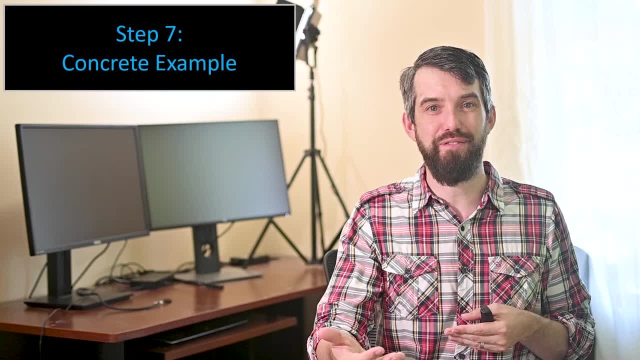 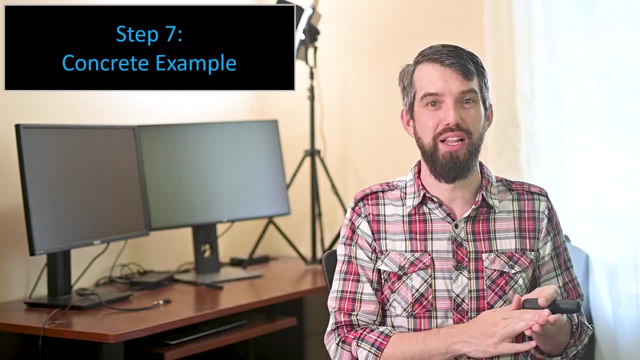 something that you know about. Indeed, anytime I'm learning a new mathematics field, if there's some new definitions, I always try to write down as many little examples as I can that explore a specific definition. Look at the idea of a basis. I just try to draw as many. 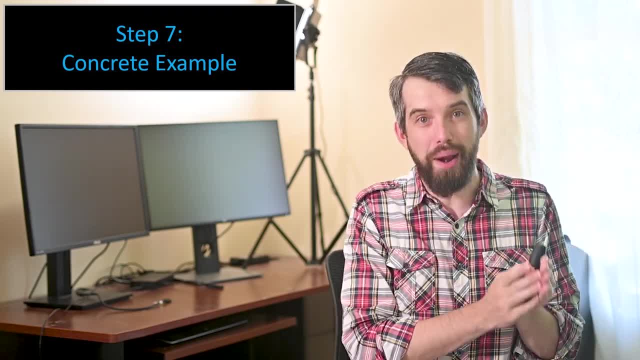 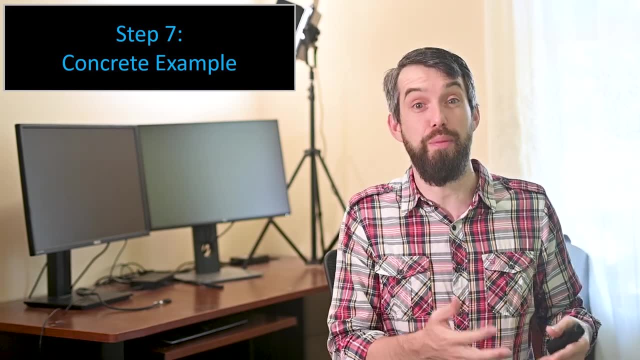 little examples of a basis until I understand what is a basis, what is not a basis. I feel that sort of doing that, exploring through canonical examples, is an extremely important part of doing mathematics- The next thing I often look for if I'm not getting any ideas. 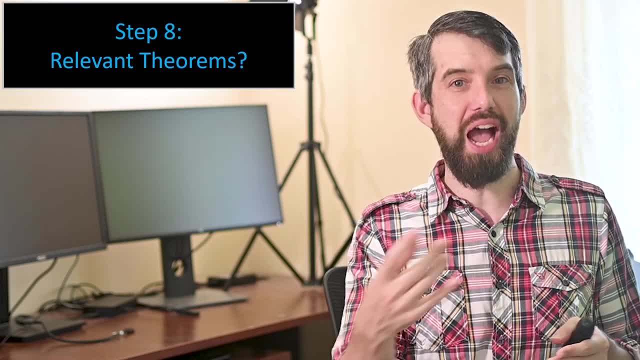 is: what are the relevant examples? What are the relevant examples, What are the relevant theorems about the kind of mathematical objects that I'm talking about? When I look at the assumptions, when I look at the conclusions, I want to know what are the major theorems that we. 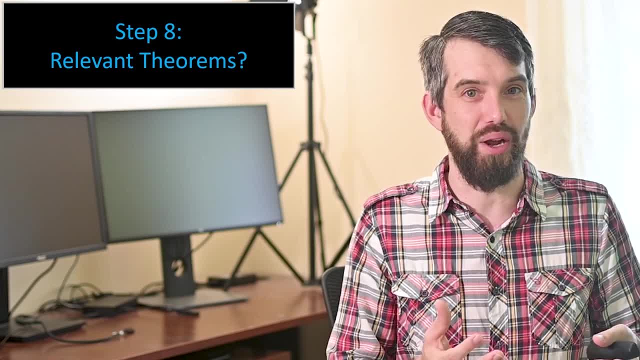 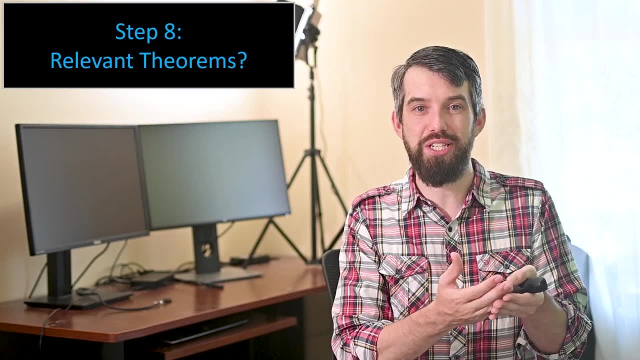 see If you're in a course. you'll often get these from your textbook and it'll be taught about in class. These are the major ideas that you need. Indeed, a lot of proofs are basically just write down the definitions, see what theorems apply. sort of connect those together to get to the 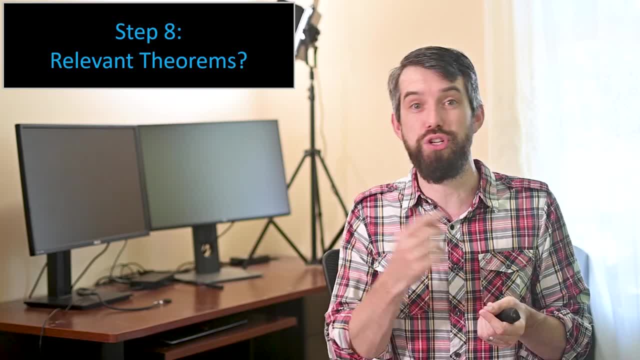 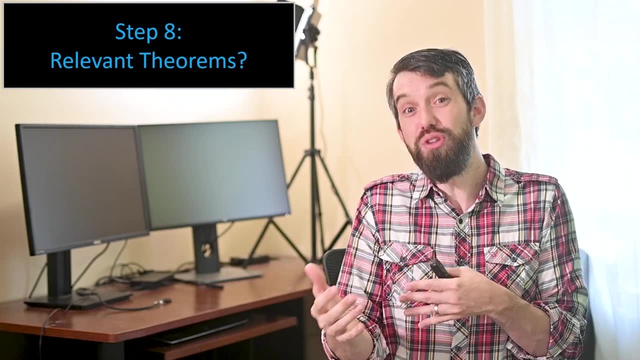 assumptions. That's sort of the core math. that's just linking one or two theorems to the definitions that you actually have. I really encourage you to sort of see what's available here. If you want to, you can even go a little bit further. This doesn't always work, but sometimes, if you read the proofs. 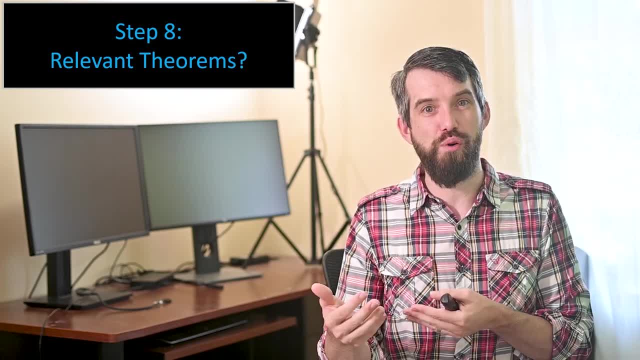 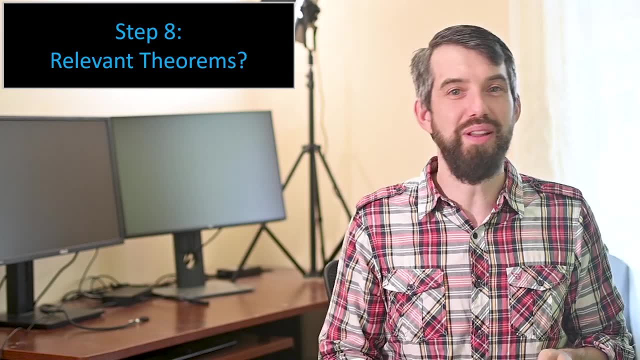 of the relevant theorems, then that can give you ideas for the types of manipulations people do with the objects that are in the theorem that you're talking about. And then the final thing I'm going to talk about is really just to sort of play around. 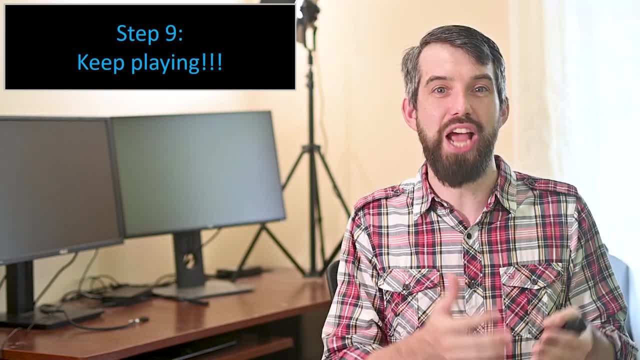 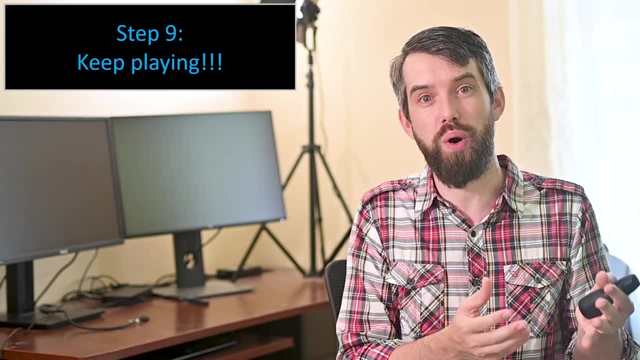 I noticed that when I was younger and I would try to prove something that I got challenging and I got stuck on. well, it would often feel a little bit discouraging. I might not want to continue. The obvious: first thing: I tried, it didn't work. Well, I'd really encourage. 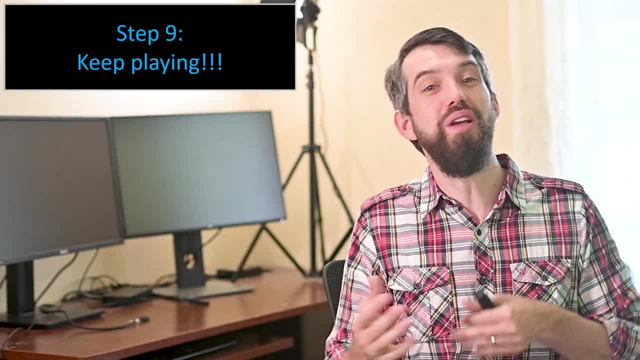 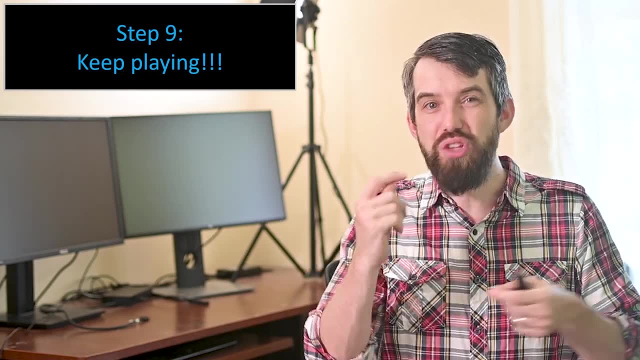 you to treat proving things as a more iterative process, where you can keep on playing around, try new examples, try new ideas, see if you can connect a new theorem in, see if there's some way you can visualize it. All these things we've talked about just keep playing around. 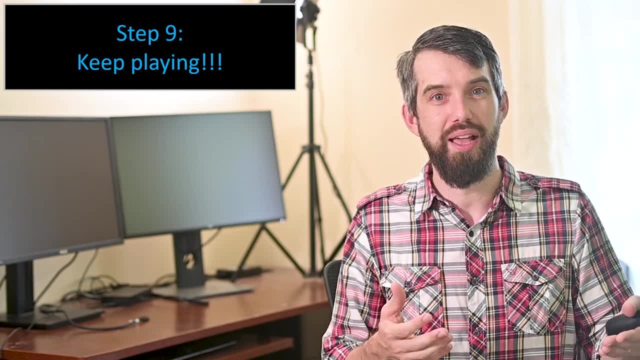 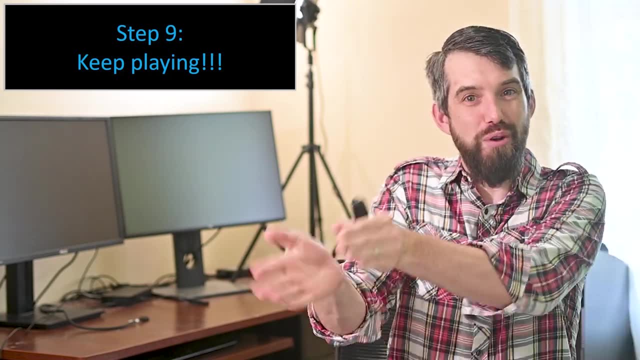 and hopefully you're going to get some insight as to how you can proceed forward. And often you find that you go down a weird rabbit hole. and you've been doing all of this, trying to do a direct proof And if you're positive, it felt really easy. So, just because one method is really not proving,